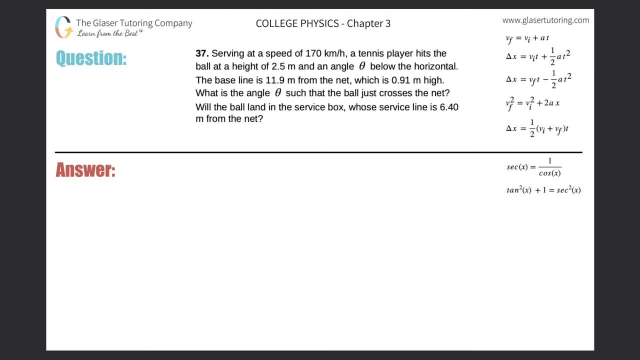 Number 37.. Serving at a speed of 170 kilometers per hour, a tennis player hits the ball at a height of 2.5 meters and an angle theta below the horizontal. The baseline is 11.9 meters from the net, which is 0.91 meters high. What is the angle theta, such that the ball just crosses the? 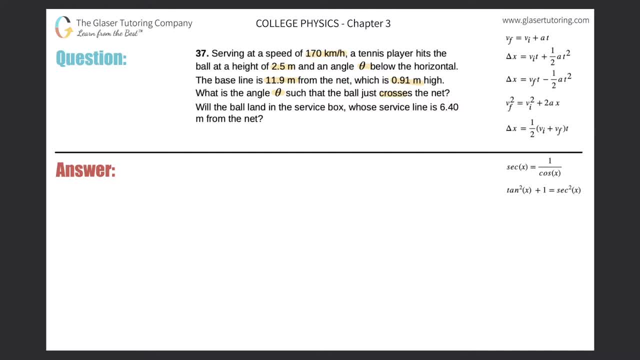 net. All right, So let's just try to draw a picture. All right. So we have a tennis player- And if that's not Roger Federer, I don't know what is- And there's the ball And he's going. 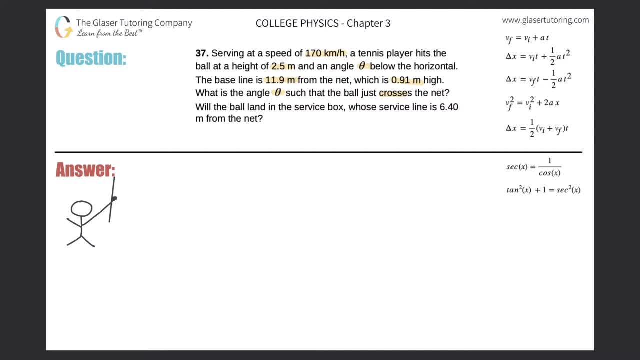 to be serving the ball. So let's draw a set of coordinates at the top. There we go, And there Now the ball is going to have. it says it's going to be struck with a net. So let's just try to draw a picture. All right, So we have a tennis player. 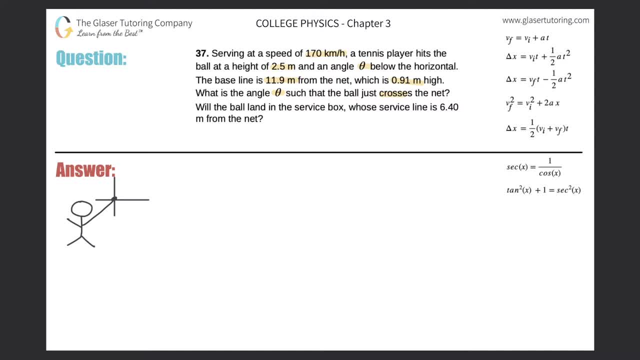 It has an initial speed of 170 kilometers per hour And that vector will be below the horizontal. All right, So we have something that looks like this, What I'm going to do. actually, instead of writing the 170 kilometers per hour here- I know it's better off we just convert it. 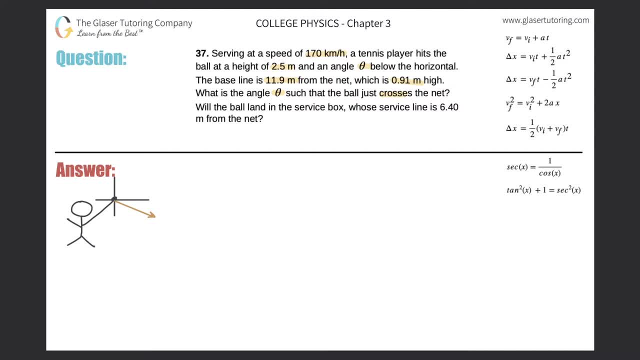 into meters per second, just because the acceleration will probably be dealing with gravity in the problem And that's in meters per second squared, So let's just take care of that right now. So 170 kilometers per hour per one hour. Kilometers on the bottom to get kilometers on the bottom, meters on the top, 1,000 meters to. 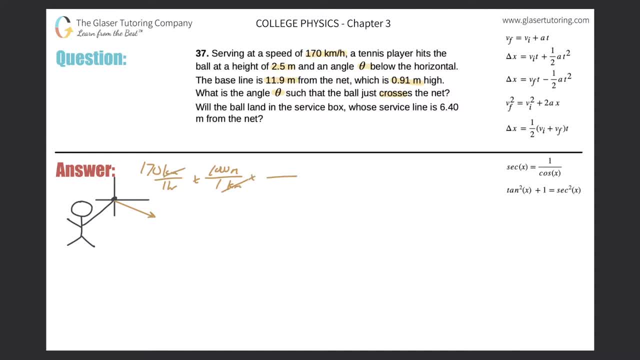 one kilometer. Kilometer goes away. Now I got to get rid of hours in the denominator, So hours go in the numerator, Then minutes in the denominator. There's 60 minutes in an hour. Hours cancel. Now I got to get rid of minutes, So that goes in the numerator And then seconds. 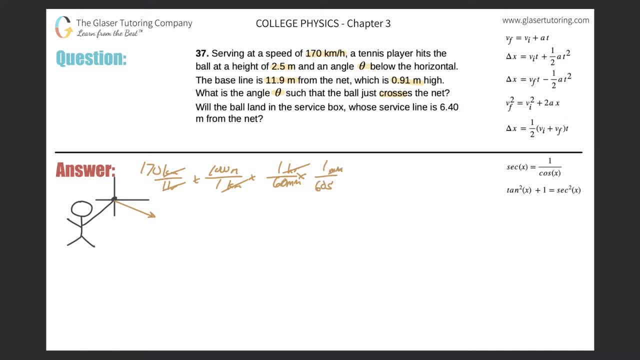 in the denominator 60 seconds in a minute, And that's our conversion. So it's just 170 times 1,000, divided by essentially 3,600.. So it's 72,. excuse me, 47.2.. 47.2 meters per second, All right, So that's going to be the value here. This is going to be. 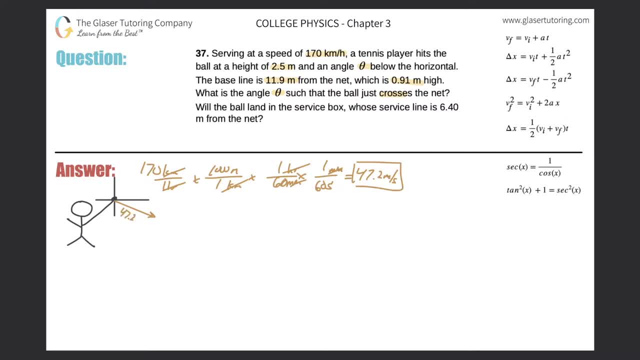 47.2 meters, And actually you know what? Let me write out that it is the initial velocity: 47.2 meters per second, Okay, great. So then there is, say, ground, right, There's a ground to this problem, Okay, And there's a net, a certain. 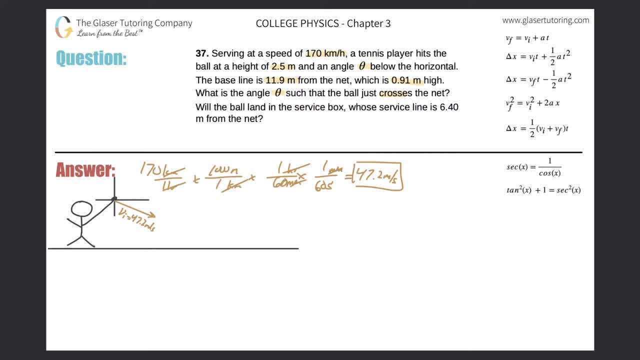 distance away right. So let's draw in the net, Let's say the net is about right, I don't know right here or so, And that distance right. the height of the net it tells us is 0.91 meters high. 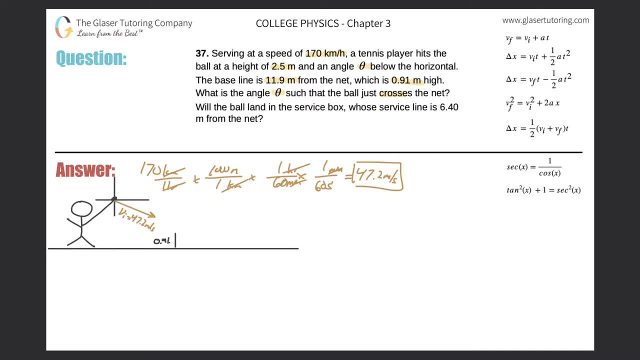 So let me write that over here. So 0.91 meters high And the net from the baseline. let's say the baseline is right here where the net is. So 0.91 meters high And the net from the baseline. 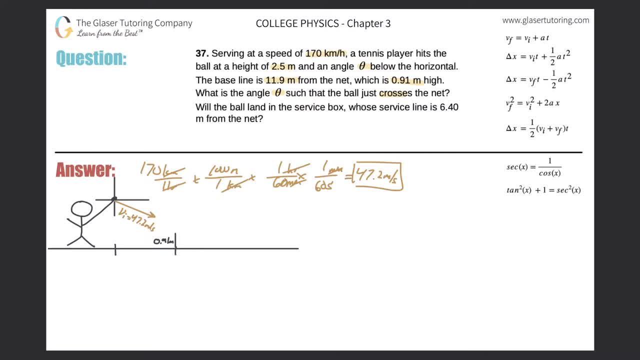 the ball is being served right. This net right here is a. the baseline is a distance of 11.9 meters from the net. So right in here now. right, we have a distance of 11.9 meters, Okay, great. 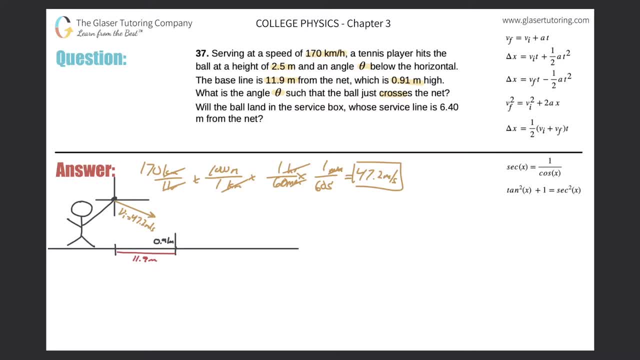 And what else? Oh, and they also tell us the height of the ball right above the ground when it's being served is 2.5 meters. right? So this is 2.5 meters, Okay, So now I think that's everything in the problem, right? Yes, it is. And what they're asking us to? 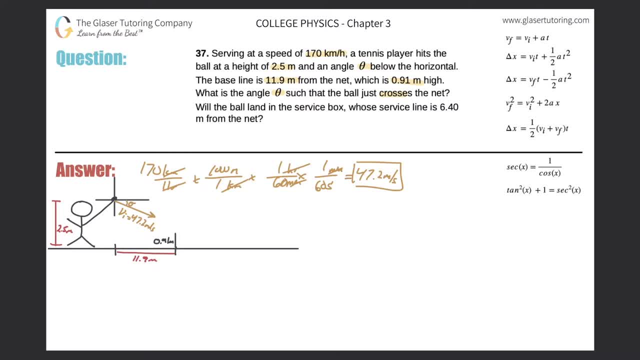 do is they're asking us to solve for this theta. Okay, So right now it almost sounds like we don't have enough information. We do, but we're going to have to do some substitutions And we got to solve some equations for variables. It's a little complex, but let's get to it. 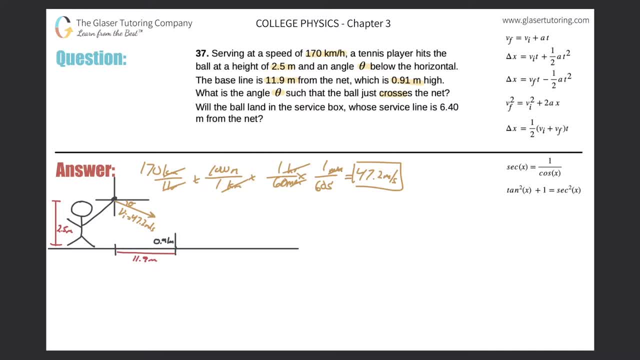 So, basically, the first thing is I'm first going to break up this initial initial velocity vector into x and y components. Why am I going to do that? Well, I they gave me a horizontal distance right And I can only take this horizontal. excuse me. 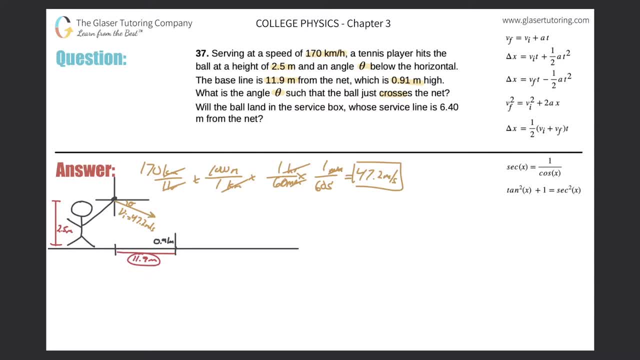 horizontal distance into account. if I find the x component of the initial velocity- And they also gave me some vertical components right- The height of the net, they give me the height of the ball And in terms of the initial velocity I can only take the y component. 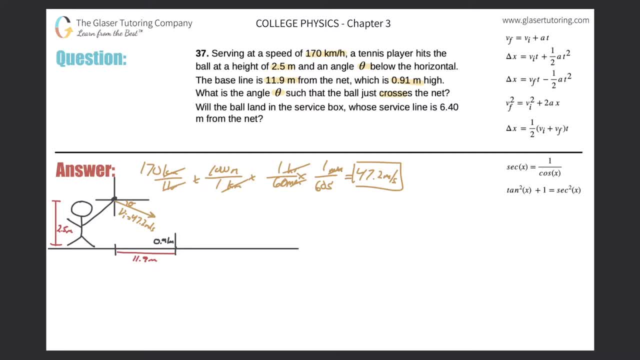 right- The initial velocity in the y direction, when I account for those heights. So let's first break that up into its components. So we have an x component here And let's let's take that to be. what would this be? This would be vi x- the initial velocity in the x direction. we don't know what that is. 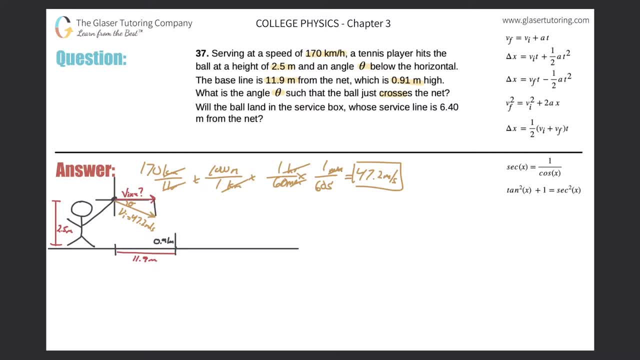 And then we will take this vector right here- let me draw it a little straighter- that vector right there that will represent the initial uh velocity in the y direction. Now just be careful here. this is going to be negative. 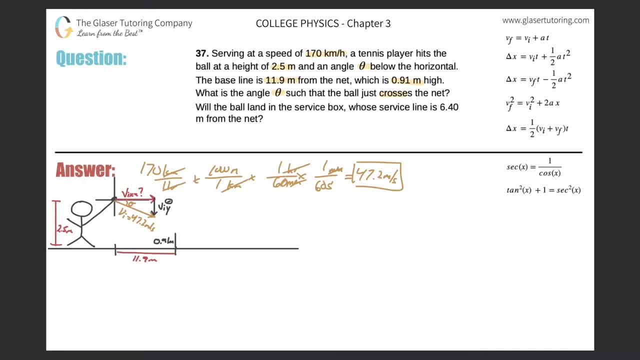 right, Because it's in the negative y direction. so we have to take that into account, all right. Whereas the x component is positive, since it's in the positive x direction, All right. so now let's just create a formula, uh, that solves for initial velocity in the x. 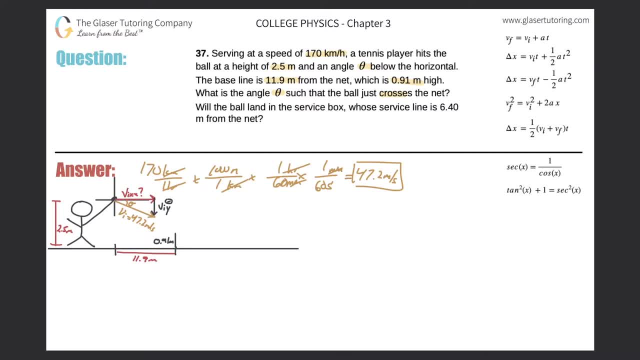 and initial velocity in the y direction. all right, So we're just using simple uh trigonometry here. We know the hypotenuse of the triangle, we know this angle and we're looking for the side of the triangle. this is the side that is adjacent to that angle. therefore, I'm going to use cosine. 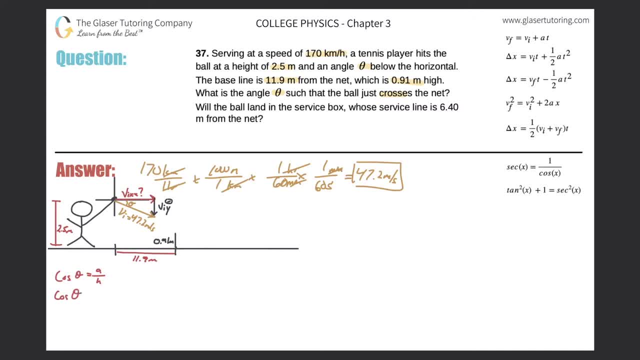 So cosine of theta is equal to the adjacent side of the hypotenuse. cosine of theta is equal to the initial velocity in the x direction right, divided by uh 47.2.. So the initial velocity in the x direction will equal 47.2 times cosine of that angle. 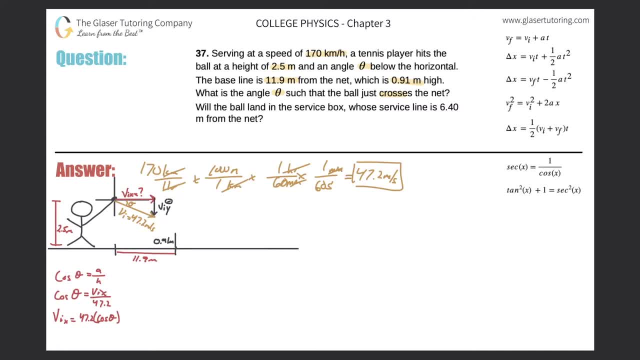 Okay, That's all. that's all I can do there. Now let's do the next exercise, the same thing for the initial velocity in the y direction. Instead, though, I'm going to be using sine, because that side is opposite of the angle. So now let's do. 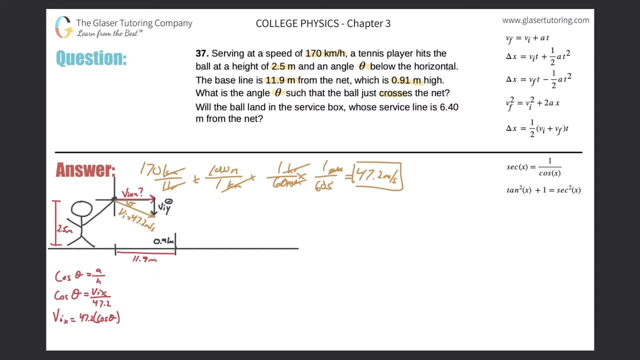 sine of theta- Actually I'm going to move it over a little bit because I think I'm going to need as much space as possible here. Sine of theta will equal the opposite side over the hypotenuse, So sine of that angle which we are. 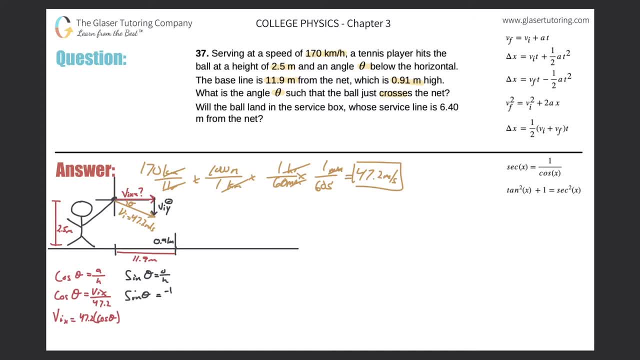 calling theta is equal to. now here's the thing: negative vi y. Why is it negative? Because it's in the down direction over 47.2.. Okay, so this means now that it would be, it would be negative vi y, right, and then that would equal 47.2 times. 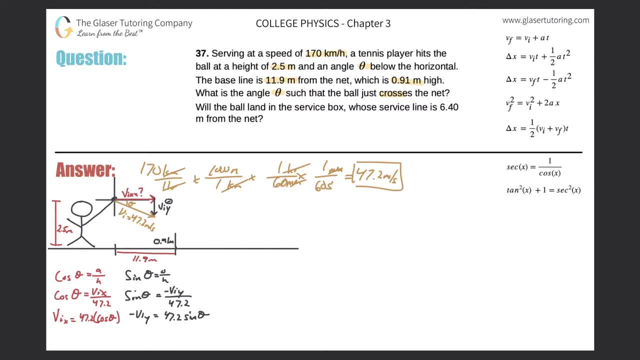 sine now of theta. Okay, great, Now, just right, I would divide this side out by minus 1.. I'm not going to do the steps because I need the space. So let's just erase this little negative sine On the left hand side and just bring it on over to the right. So that's negative. 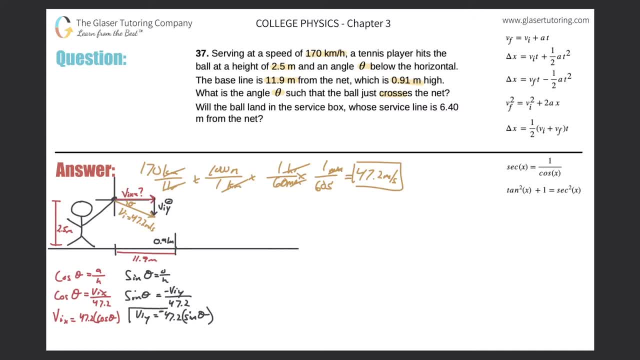 Okay, so we have these two, these two equations, here, Okay, great, Let me just box this one, Alright now. so we got that out of the way. Now let's try to do something with this particular distance. Alright, this is a horizontal distance, so 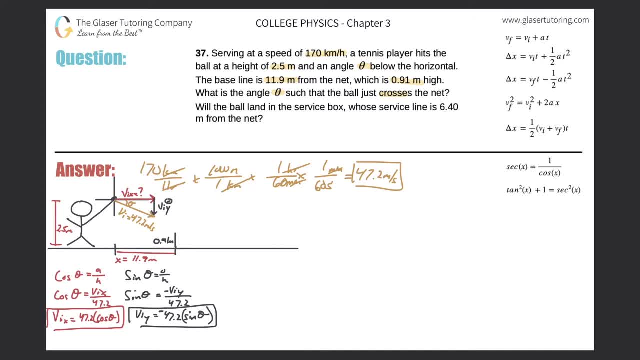 therefore it's an x component, right, it's an x displacement. And now remember, in a free-fall problem, because essentially, once the ball is struck, it's a free-fall problem. there are no accelerations in the x-direction, Therefore the velocity is constant. the entire problem in the 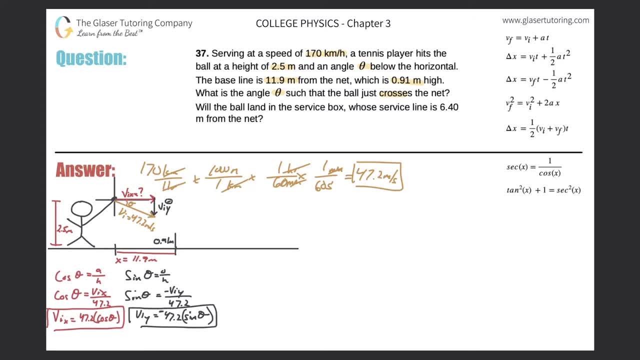 x-direction. So, that being the case, whatever initial velocity I found here will be the same velocity everywhere in the problem. Alright, so I can say that velocity will equal the displacement over time. Now, specifically, right, I could plug in the initial velocity here, because velocity in the x-direction 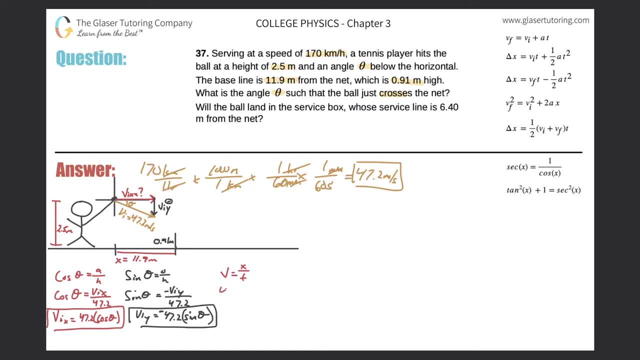 again is the same. So that's what I'm going to do. so I'm going to do forty seven point two cosine of theta, alright, will equal. then 11.9 over t, Alright, let's leave that alone, Right? so now what I'm trying to do is I'm just 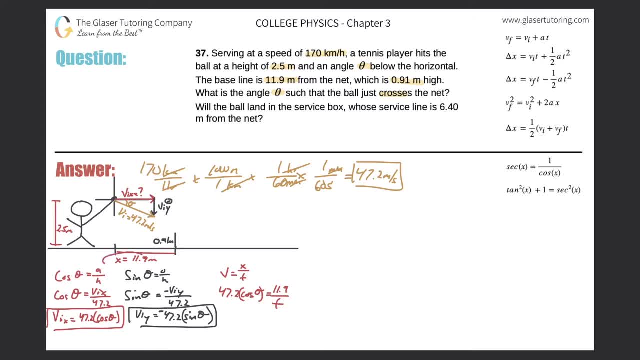 trying to incorporate the. why did I do that? I'm just trying to incorporate more information into my formulas. Alright, now that's all that we can do for x. that's it Now, the only other thing we can do now for y. remember they the other. 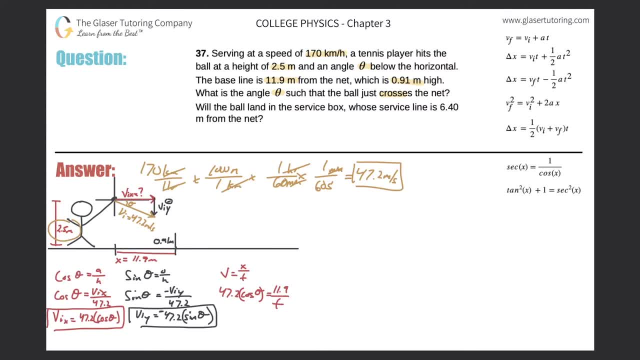 information they gave us was in terms of heights. so they gave us the height of the ball initially and they gave us the height of the net right. so, if we picture it, this ball is going to travel right and then it's going to come down at some angle like that. so we want to make sure that the 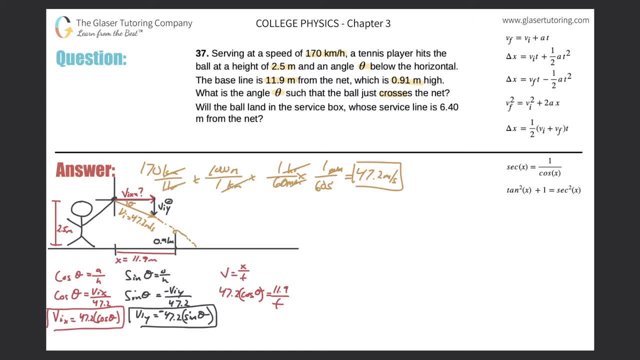 ball just passes the net there. okay. so, if we think about this, if i, if i call this my initial state of conditions for the um, for the y calculation here, and this point my final state, okay, what do i know about these conditions, about these, uh, frames, about these states? well, what's the displacement? 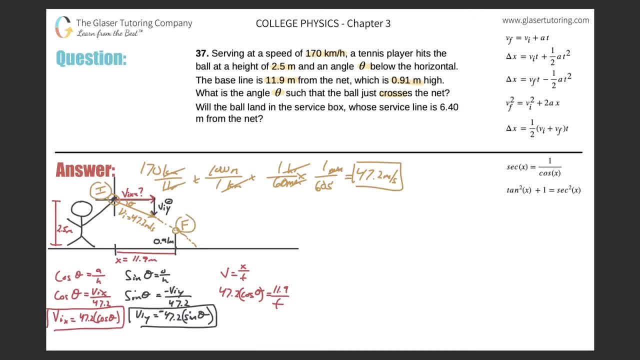 between the initial state and the final state here. how could you calculate that? well, it's easy, right? if we were to think about: how do we calculate? uh, displacements, change in displacements. we calculate the initial state of the ball and the final state of the ball and the final state. 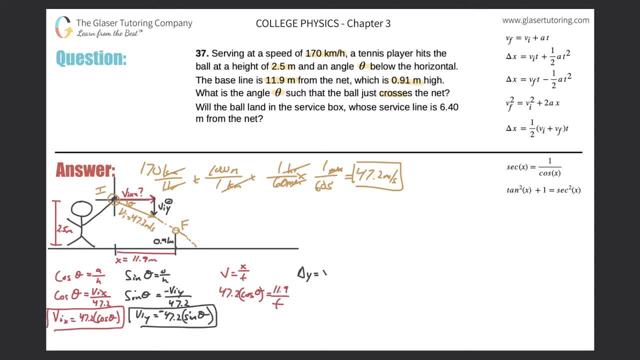 by doing this right change in the displacement of y will equal the final value of y minus the initial value, right, minus the initial height. okay, so what is the final height? if i call this point my final point? well, that would be 0.91. and what's the initial? well, if i call that my initial point. 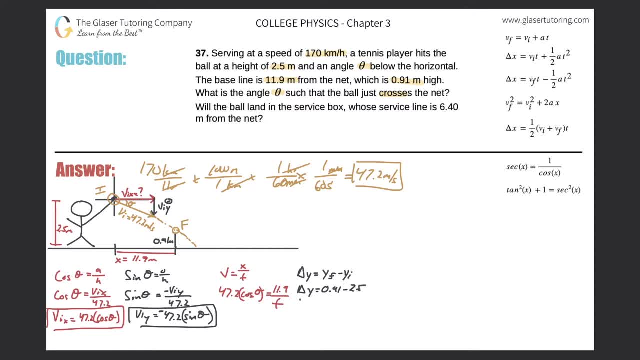 the initial height was 2.5, so 2.5 great. so now i can find my change in y value, so it's 0.91 minus 2.5 or negative 0.59, but we're going to round to negative 1.6 and that's in meters. okay, so that. 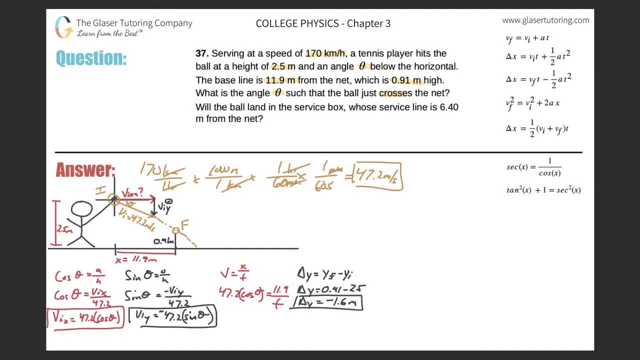 i found there now, in terms of this frame, from the initial frame to that final frame. what's the acceleration? remember we're talking about y, so therefore it is gravity negative 9.80 meters per second squared. all right, do we know the final velocity in the y direction? uh, no right will it? 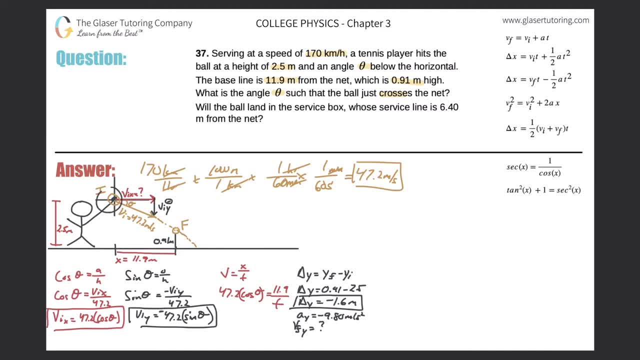 be same as the in the final velocity in the y direction? no, right. will it be same as the in the final velocity in the y direction? no right. will it be same as the in the initial y velocity? and no, because it's falling right. so since there's an acceleration in the y direction, that that. 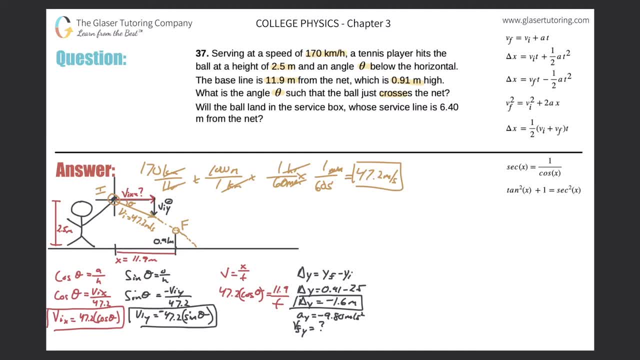 velocity should be changing, so it won't be the same as the initial. it'll be different. remember, we already found a formula for the initial, okay, and now, the only thing that i don't know about this is time, correct. but here's a thing: time is a little special, right? um, the reason being is: 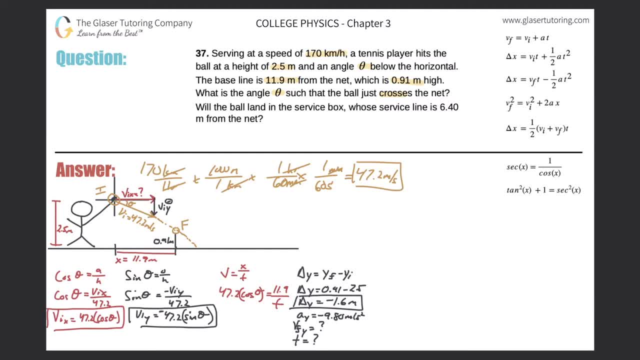 because time is component less meaning. time is a little special, right. so time is a little special time. there's no component to to it. there's no such thing as x time or y time, it's just time, right. time knows no boundaries, it knows no difference between the x and y coordinates, and therefore 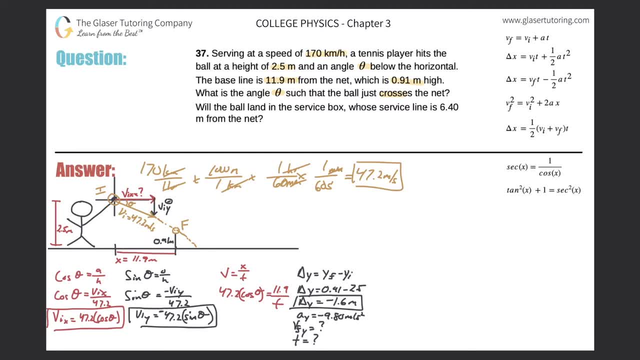 time is an important variable in these problems that allow you to connect x frames or x components with y components. okay, you can't do that with the other variables because they're all in different dimensions. right, they're all in one is in an x dimension, one's in the y dimension. 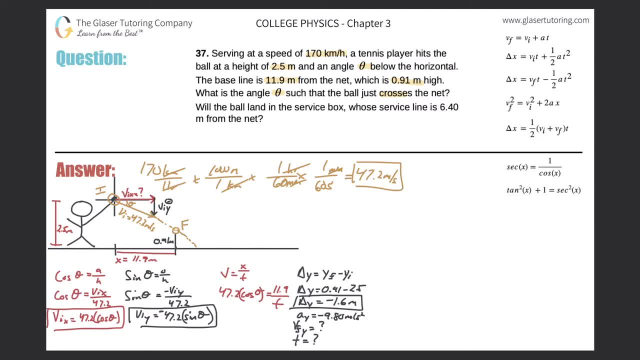 so. time, though, knows no dimension, so what i want to do here actually now, at this particular point, is: i realize i created a formula here that has time in it. now i'm thinking to myself: well, wait a minute, if i can now create a formula with all of these givens and knowns and unknowns, 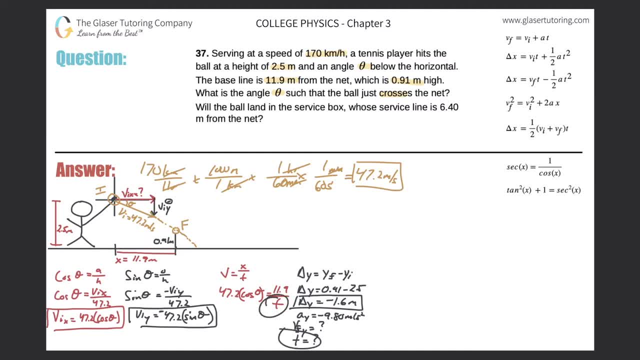 with time in it, maybe i can start substituting things right and maybe that'll get me somewhere. all right, because i definitely don't have enough information right now in terms of these formulas to solve. i gotta do a whole bunch of substitutions. so what do we need to do? well, i need to use the 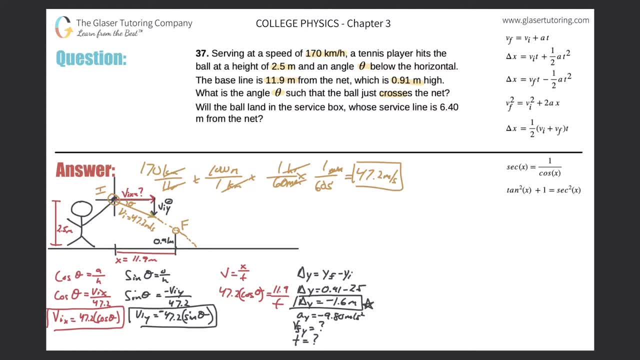 displacement, right, the displacement, and y because that's additional information that they gave me. in the problem i need to use acceleration and i also want to remember the whole goal is to try to solve for theta here. all right, so maybe i want to include a formula with my initial velocity in the y. 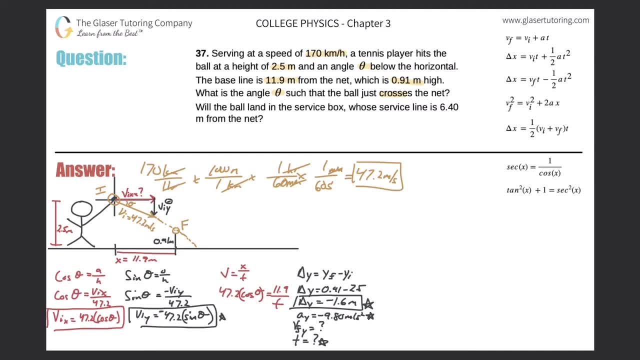 direction. all right, and maybe also then time. i definitely want time in it, because then i can connect these two equations together. so which one are we going to choose? it sounds like number two. in the upper right hand corner fits the bill here. so when i do that, let's see what happens. 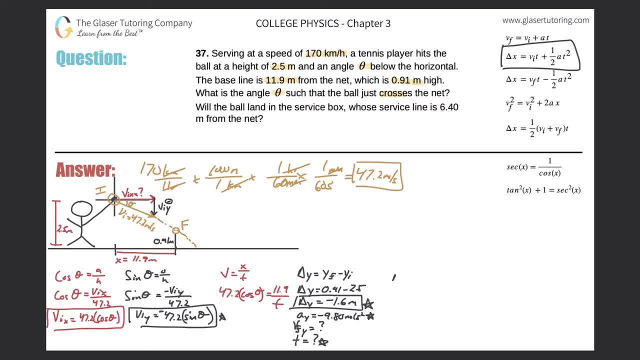 so what i'm going to do is: um, let's write now. change in y right is equal to the initial velocity in the y direction times time plus one half of the acceleration in the y direction, times time squared. so the displacement or the change in y right was negative, 1.6. 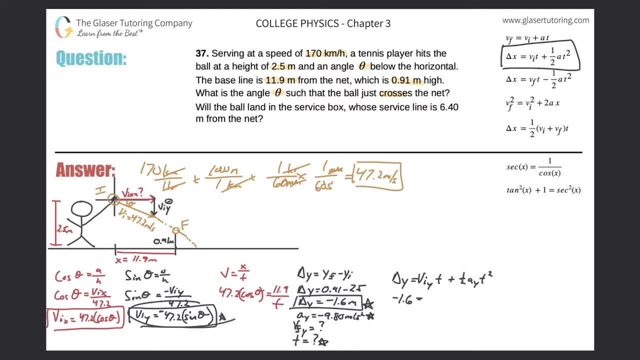 the initial velocity in the y direction is what we found over here, right? so that's going to be negative 47.2 sine of theta. okay times time plus one half times the acceleration in the y, which is negative 9.80 times time. squared, all right, great. let's just clean this up slightly. not really too. 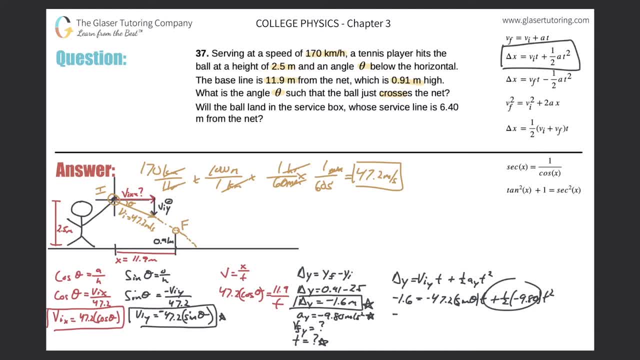 much to clean up here, but let's just combine these terms essentially. so we got: negative 1.6 is equal to negative 47.2, sine, oops, sine theta times t, plus now half times negative 9.8 is going to be uh negative. so actually let me just get rid of the plus sign. negative 4.4.9, t squared okay. 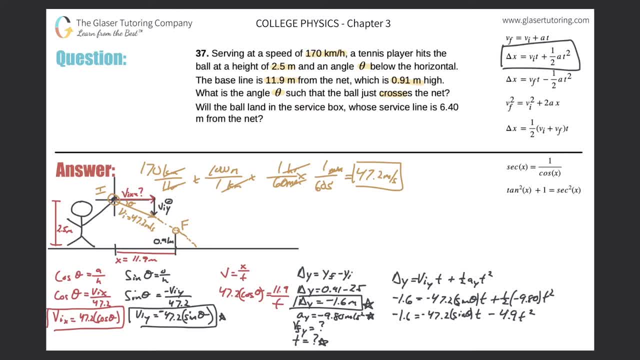 now, what do we want to do? well, now, look what we have, guys. we have this equation that has two unknown zes meaning theta and time. and now I just created another equation that has two unknowns also: theta and time. well, that's wonderful, right? because now I realize I have two equations with two. 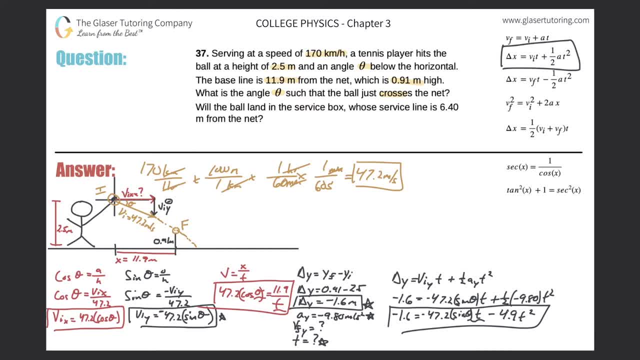 unknowns. uh, that that's a solving system of equations now, meaning that all I have to do now is solve one of them for, let's say, time and then plug it into the other equation, and now I'm going to start to get an equation, then, with only one variable. 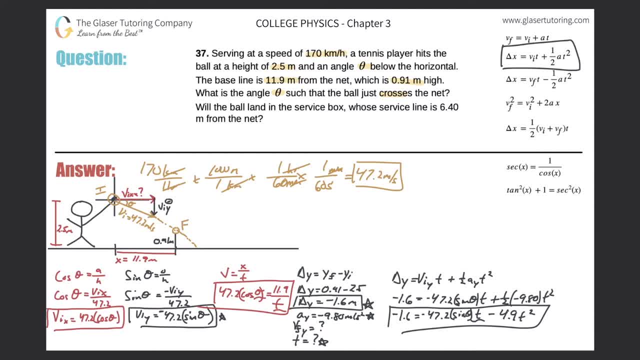 And that's what we like, because if we have an equation with only one variable, we can solve it. We can solve that All right. So let's now take this equation right here and let's solve it for time. Basically, just switch the numerator and the denominator. 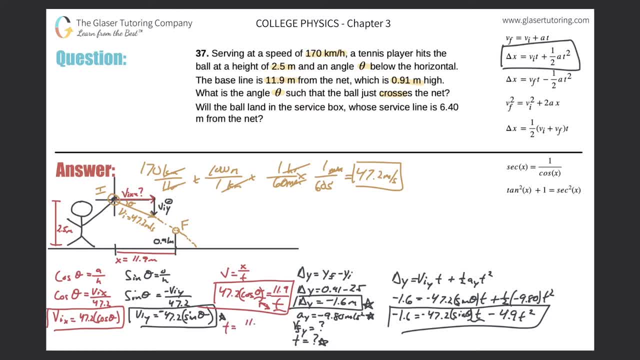 Okay, it's a little math trick. So time will be equal to 11.9 over 47.2 cosine of theta. Now what I'm going to do is, since this is equal to time and the time in the X frame is the exact same thing as time in the Y frame, doesn't matter. 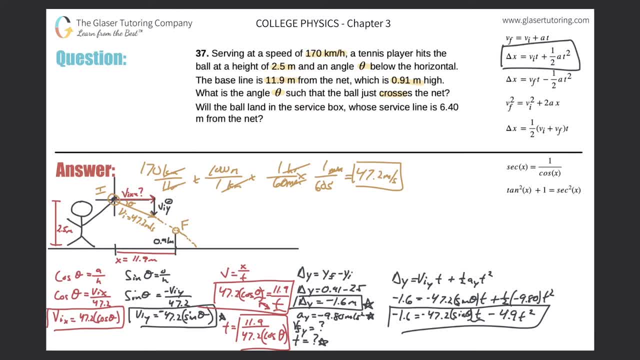 Okay, And also remember well, not only are they the same time, but we're talking about the same points, right? Because my X dimension, my displacement in the X, was 11.9.. Notice how that distance correlates with this being the initial point, which is essentially on the same plane as the initial point for Y. 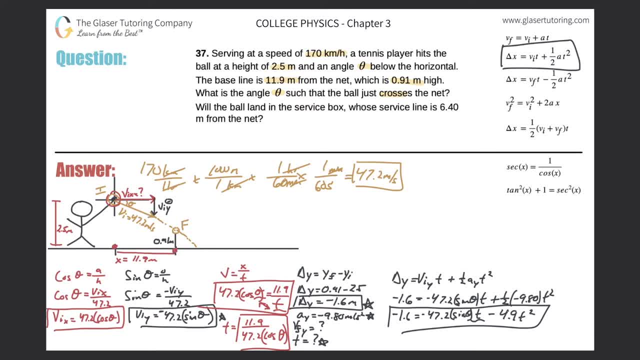 And then it talks about this being the final point, which is also the final dimension for Y that I chose. So that's why we can do this All right. So let's take this thread, the needle, here And now. what we're going to do is just plug it in for time here and time here. 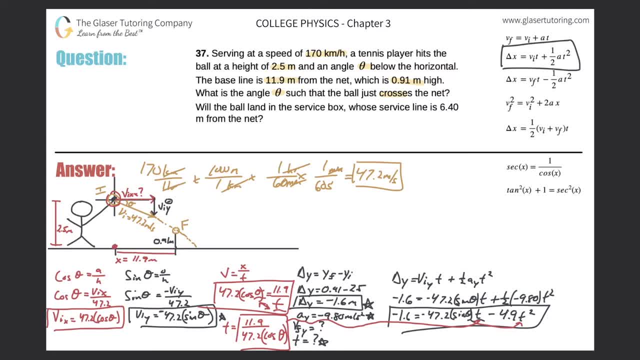 Okay, So what I'm going to do is I'm going to rewrite it at the top, All right, So let me erase this conversion stuff, All right, That's not really important anymore And let's try to see. Let's see what we can write on the top now. 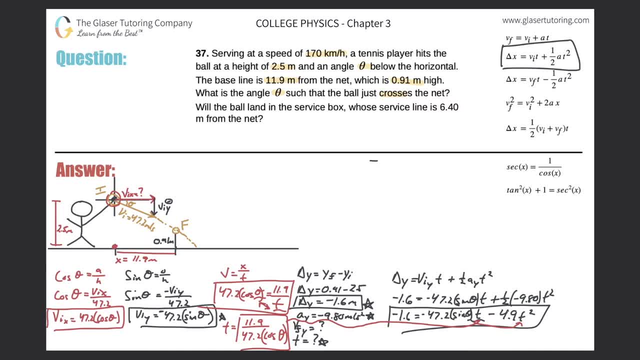 So my formula is going to become now negative. Let me give myself some room. Right here should be good. Negative 1.6 is equal to negative 47.2 sine of theta times time. But instead of time I'm going to plug in the 11.9 divided by right: 47.2. 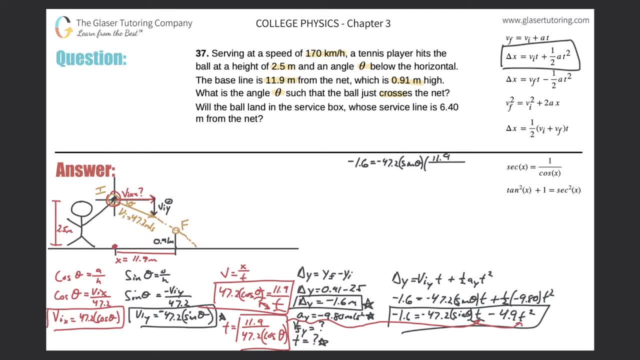 So now it's going to be 11.9 over. Oh, I don't, I didn't give myself enough room at all here. Sorry guys, Just give me one second, Apologize. All right, Let me back it up. 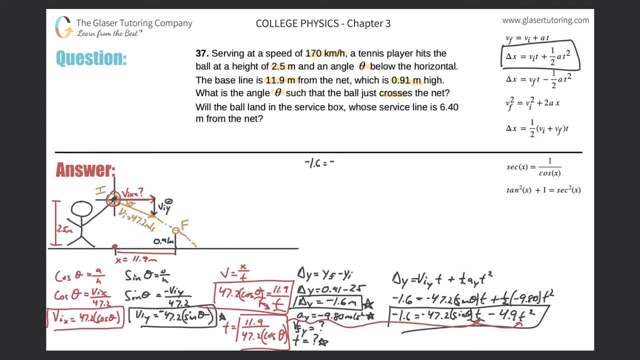 So negative 1.6 is equal to negative 47.2 sine of theta multiplied by time. But now I'm going to plug in the 11.9 over the 47.2 cosine theta. Okay, Minus now 4.9 times the. 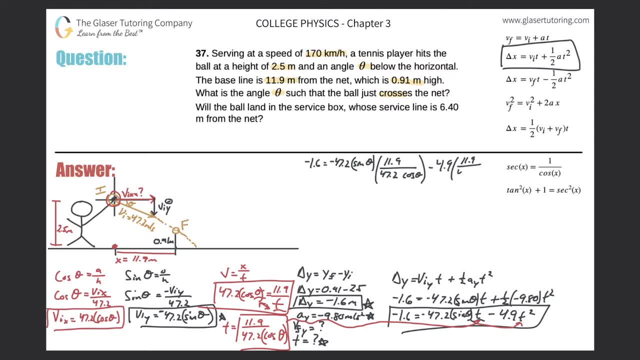 Time value squared So it's 11.9 over 47.2 cosine theta And that whole thing is squared. Oh my goodness, Right, All right. So let's see what we can do here. Let's clean some things up. 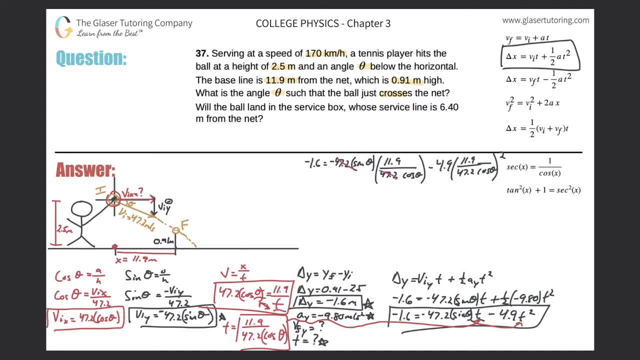 So if I notice already, I can cancel this 47.2 with this 47.2.. Right, So let's do that. So we got negative. 1.6 is equal to now negative. Let me put the number first: Negative 11.9.. 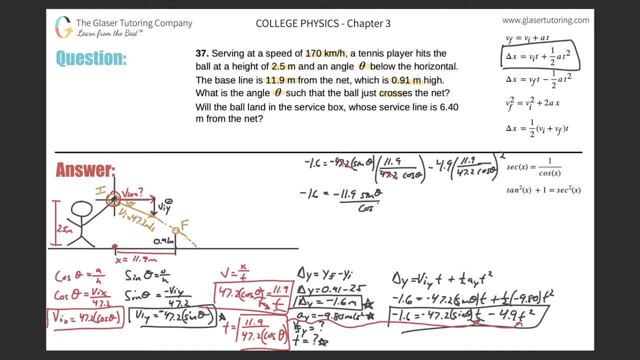 Sine of theta over cosine of theta. Okay, That, and now minus. So let's do, let's do the math here. So let's do 11.9.. So let's do 11.9 divided by 47.2.. 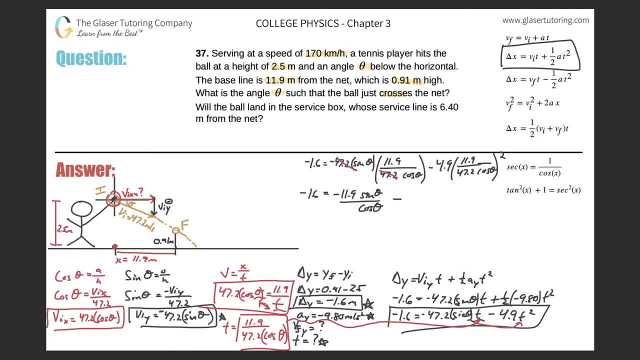 And we get 0.252.. All right, So negative 4. 4.9 times. Now it's going to be negative 252.. Well, it's not negative. What am I talking about? 0.252 all over now. cosine of theta. 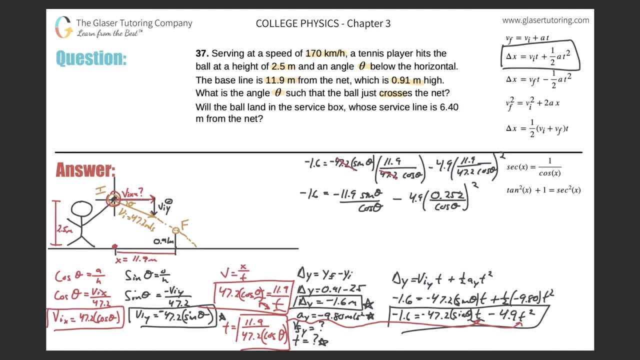 And that's going to be squared. Okay, Now what I want to do here. I want you to notice something, guys. Look at the sine theta over cosine theta. Do you remember what that is equal to? If you remember back to trig, well, that is equal to tangent. 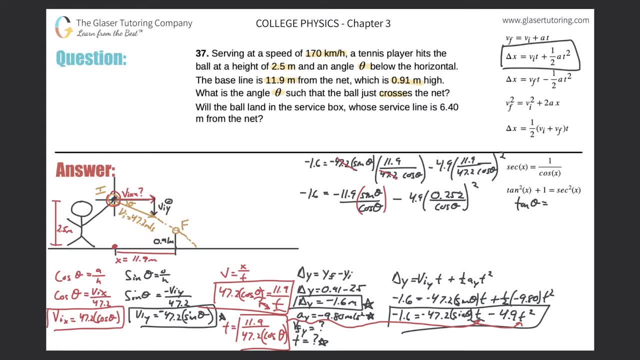 Okay, So I'm going to write that over here. So tan of theta is equal to the sine of theta over the cosine of theta. All right, We're going to have to use that. All right, This problem is very tough. We're going to need a couple of trig identities. 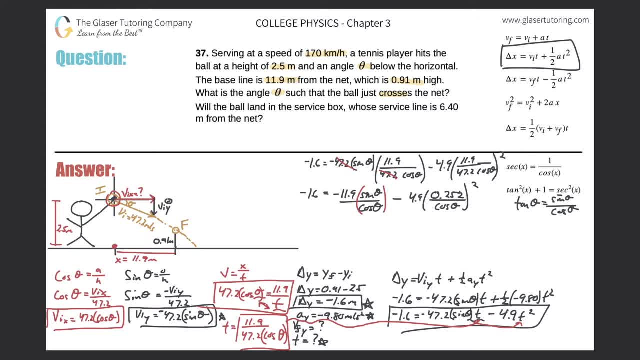 I added some to the table, some to the page on the right-hand side to begin with, But I wanted to see if you guys remembered that one, Because that one you should. The other ones are a little, not less common, but usually they're not utilized as much. 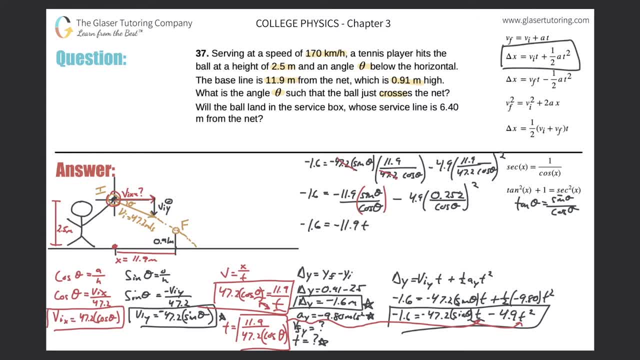 So negative 11.9. instead of writing sine theta over cosine theta now, I'm going to write tan theta. Okay, Minus now. So let me do some math here. All right, What I'm going to do is I'm going to do a little bit of math here. 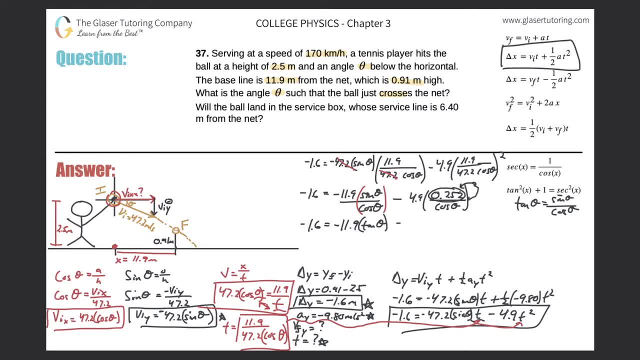 I'm going to square. Basically, I'm going to distribute the square to the numerator and the denominator. Okay, I'm going to do a, so let me take the numerator here and square it. All right, So it'd be 0.252 squared. 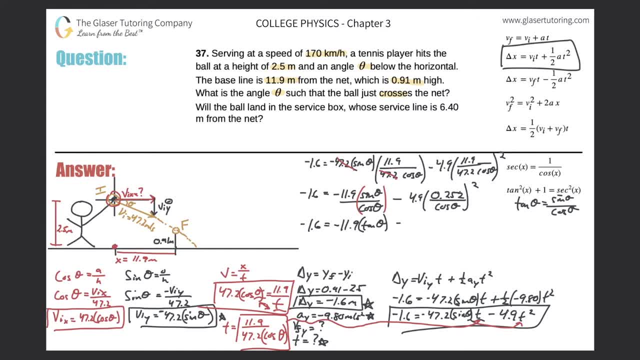 And then what I'm going to do is I'm going to take that value and multiply it by the 4.9.. And I get negative 0.311.. And now that's over cosine theta Square. All right, Let me make that square a little bigger. 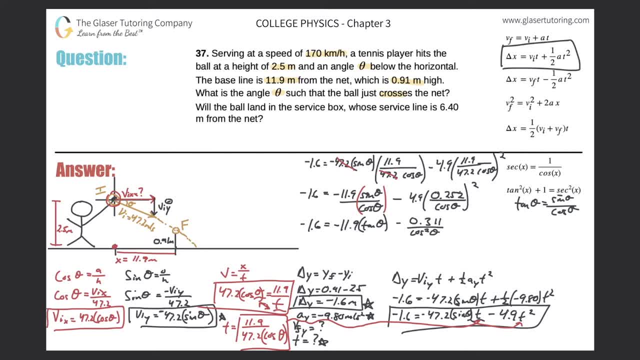 Squared. Okay, All right, Now we're good. We have one unknown, but we have two trigonometric functions. So now what I'm thinking about is how the heck do I get rid of either tangent or cosine squared? Well, I want to make them all have the same function. 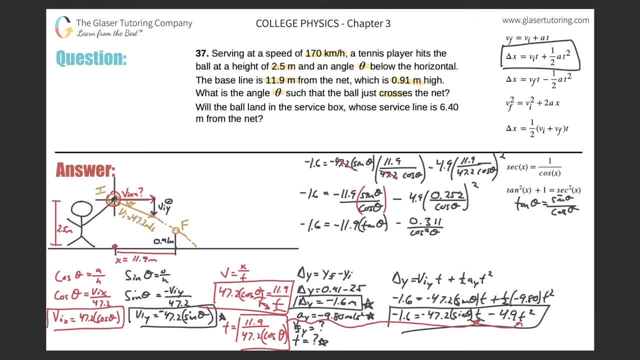 So notice this handy- Well, not handy yet, Let's. the other one's a little more handy, but this one will get us there. So notice that, Okay. So cosine, one over cosine is the same thing as secant, And this item here, basically, can be broken down into 0.311 times one over cosine, squared theta. 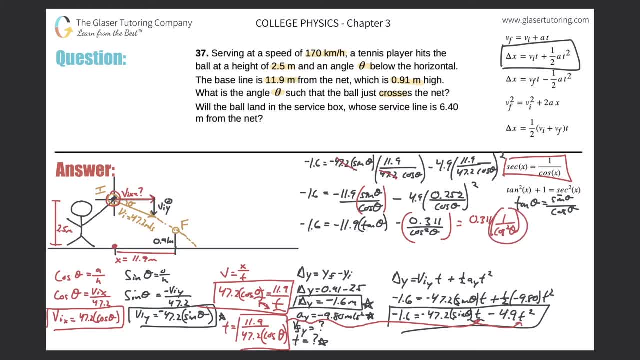 Right, That's the same thing. So what I can do here is pretend that this piece is the same as secant, because I know this relationship, All right, But now, well, it's not the same as secant, It's the same as secant squared. 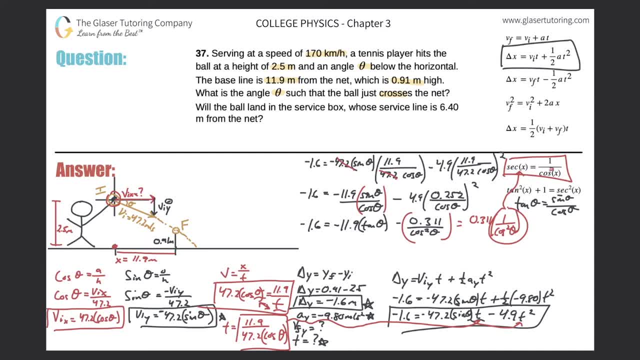 Right. So really, what I can do is alter this And say one over: cosine squared is the same as secant squared. All right, So that's what I'm going to do here. So let me just backtrack. Okay, I'm just going to put a little squared sign up there. 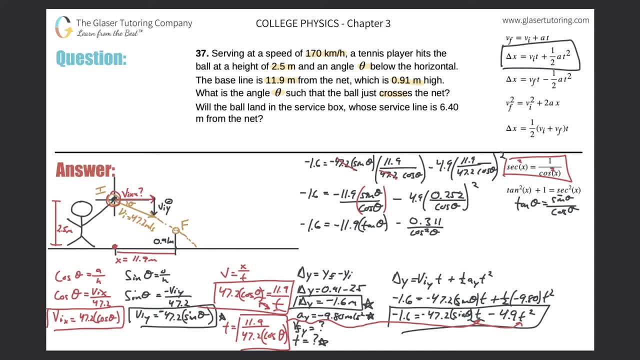 It's still valid, All right. So now let's see what we come up with here. So we got: negative 1.6 is equal to negative 11.9 tan theta minus now 0.311 secant Square theta. Now, why did I do that? 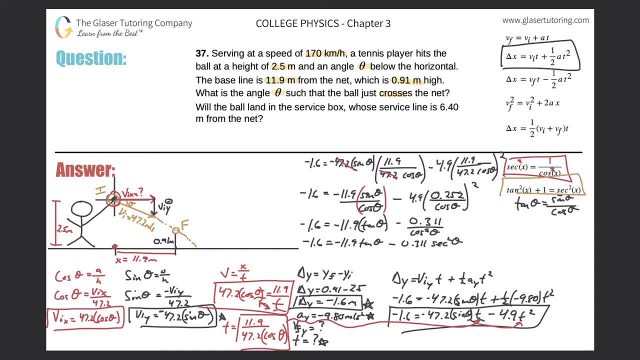 I did that because I want to use this second one now. Look at this: Secant squared theta is now equal to tangent squared plus one. That's great. Now I can finally get one equation with one unknown and one trig function. Thank God. 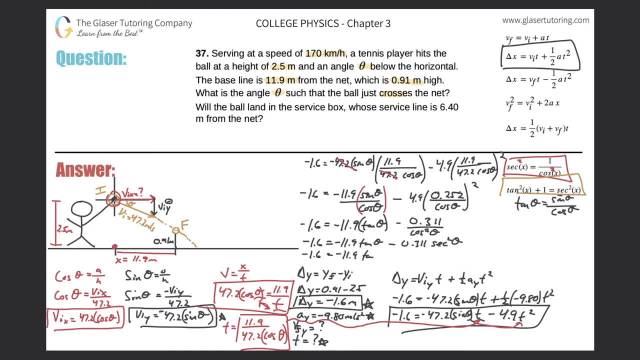 All right, So now this is negative: 11.9 tan of theta minus 0.311 times 10.1. Times tan squared theta plus one. Okay, Now, all I want to do is just do a distribution here, And now we're going to start setting this thing up. 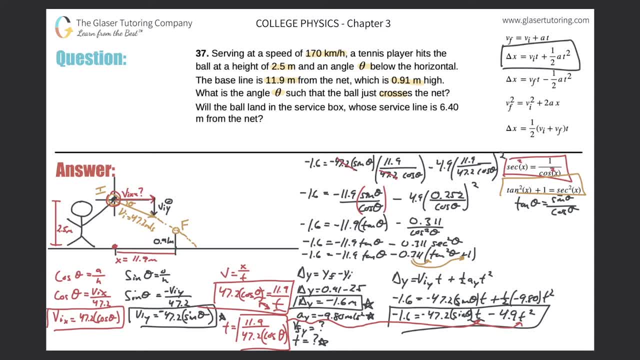 All right, I'm just going to do the distribution And let me do that. Let me do that over here. I think I might be able to fit it, So let's see. So now we're going to have: negative 1.6 is equal to negative 11.9.. 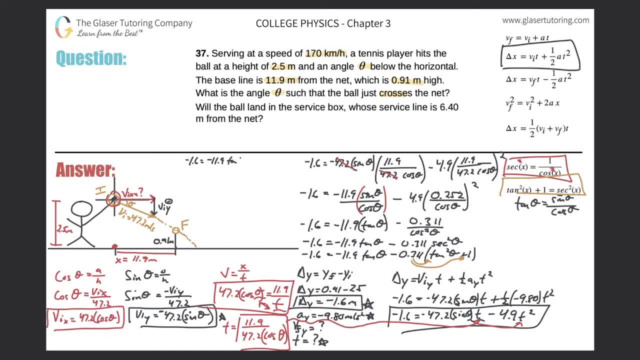 Negative: 11.9 tan theta, Tan, theta And minus. now I'm going to run close: Minus 0.311 tan squared theta, Right Minus. Let me just draw a little line here, Sorry guys, Okay. 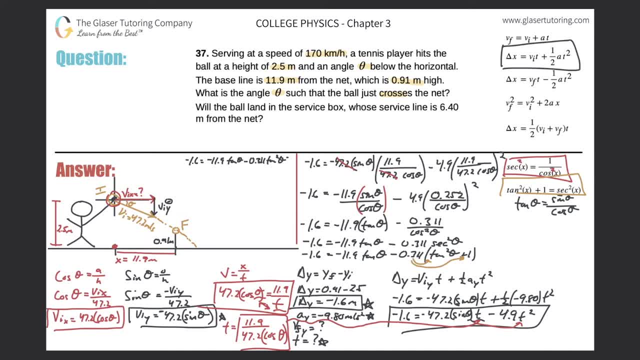 That looks good. Minus, then Hold on one second. You know what I'm going to do. Do a little magic here. Watch, There we go. Now I have enough room, Okay. So then that's going to be, And let me just erase that little piece right there. 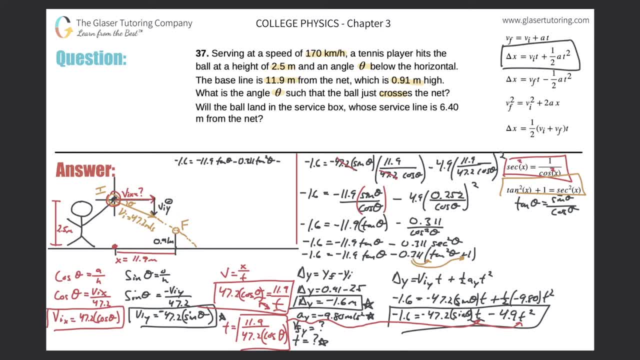 So now we have- Let me just make sure- So now we're going to have then minus, Because it's a negative 0.311 times one Minus 0.311.. All right, Perfect. So now, what do we have here? 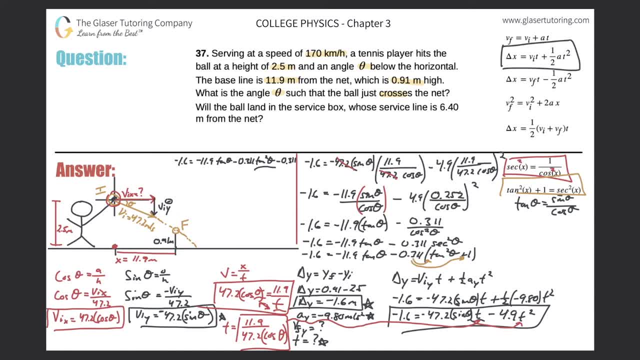 Well, now I have almost what looks like a quadratic. Right, I got a term, I got a singular term, And then it looks like I got some constants. So what I want to do is I want to try to put this into quadratic form. 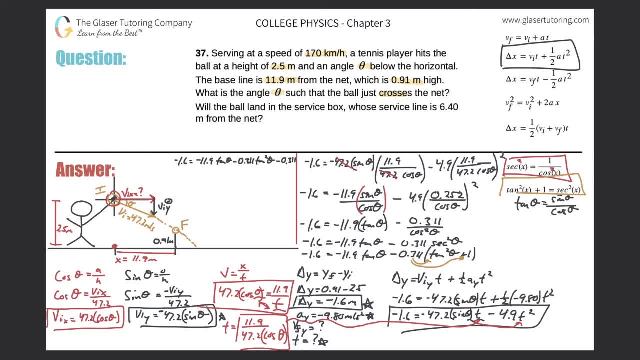 I always like having positive coefficients, by the way. So what I'm going to do is I'm going to add this term right over to the left. I'm also going to then add this term on over to the left, And same thing here. 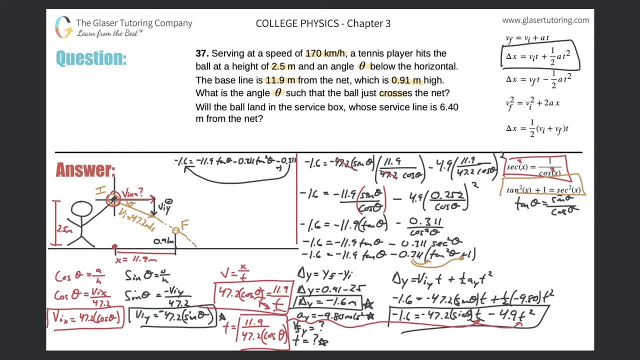 I'm going to add this thing on over to the left and combine it with its like term right there. All right, So now when I rework this, It should work out to be negative: 0.311 tan squared theta plus 11.9 tan theta. 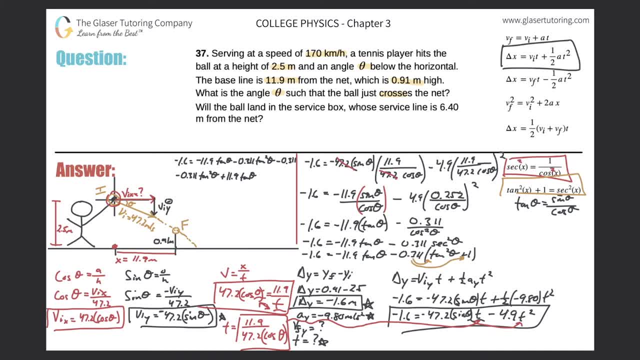 Now we just have to do some math. So it's a negative 1.6 plus 0.311.. So we get a negative. Let me just make sure I did that. Yep Negative 1.29.. 1.29.. 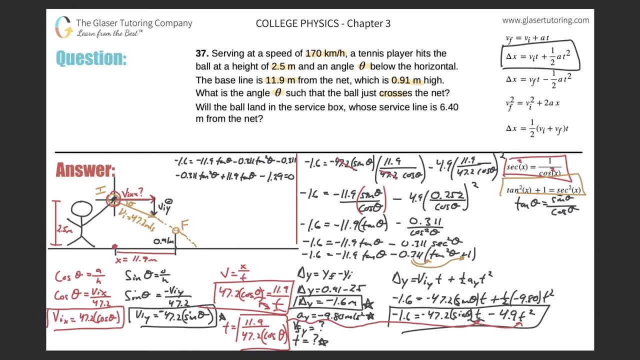 And that is all equal to 0.. So now, here is the quadratic. basically, You might say, well, wait a minute, Where's the x? I got tan squared. What is going on? No, no, This is the x. 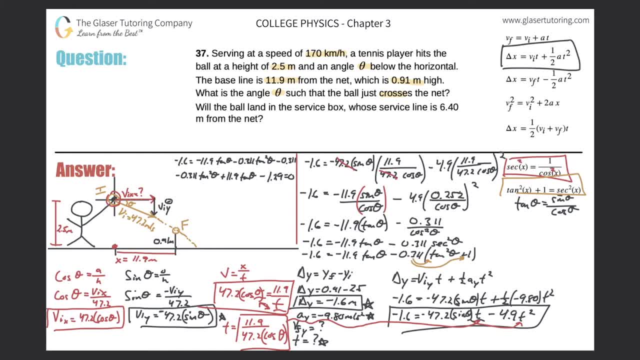 This whole thing is like x All right, So watch, This is my. Oh, I made a mistake, I just see it. So many things going on. I made a mistake. I know a lot of you are probably yelling at me right now. 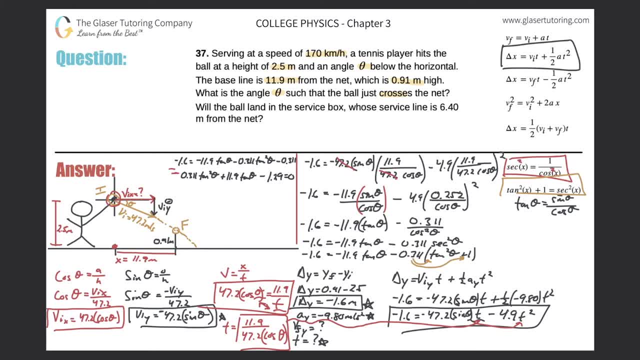 But that was the mistake, right. I had a minus sign right here, guys. I just erased it. All right, That should not have been a minus sign, It should have been a plus sign. So I'm always constantly trying to check the work as I'm looking. 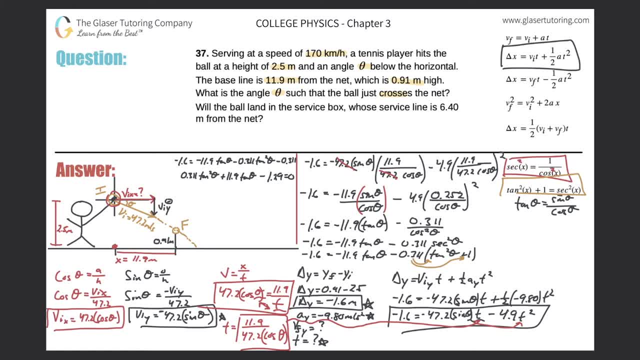 And I, At least, I caught it. So this now has the form. Let me change the color. This now has the form of a. This is my x. now, Tan theta is the x, And that's squared. Then this value right here is my b. 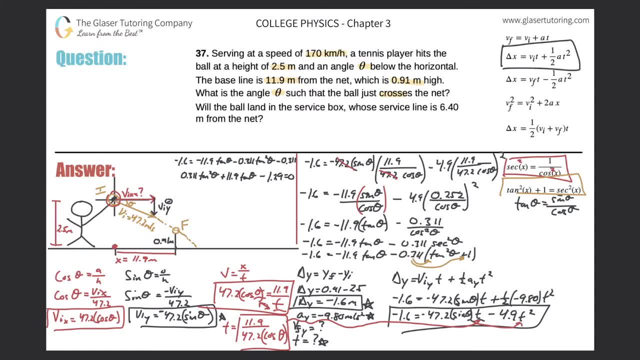 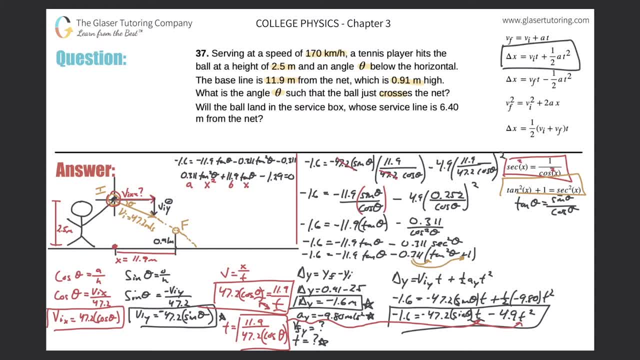 And this is my x, And this is my x, And that's my x, And this is c. Okay, So here's the a, Here's the b, And it's There's the c. So now you can use your quadratic formula. 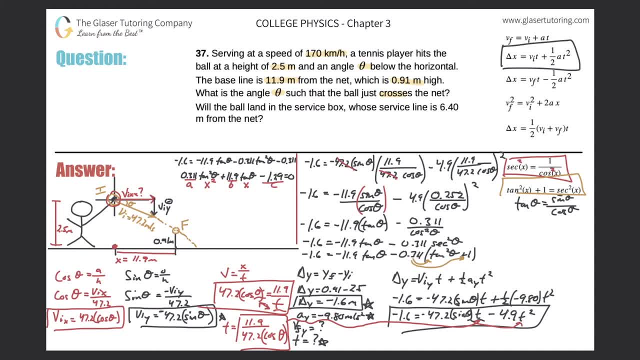 Right That Um X is equal to negative b plus or minus the square root of b squared minus 4ac, all over 2a. I'm not going to do that, You can do that, But I'm just going to plug it into my calculator at this point. 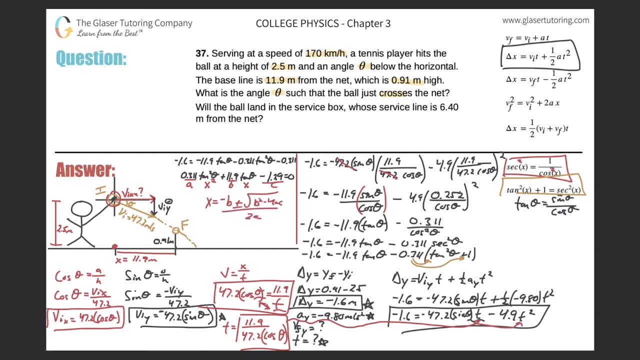 All right. So just know that the Um, That my a value here is 0.3.. So I'm going to plug it into my calculator at this point, All right, So just know that the Um, That my a value here, is 0.3.. 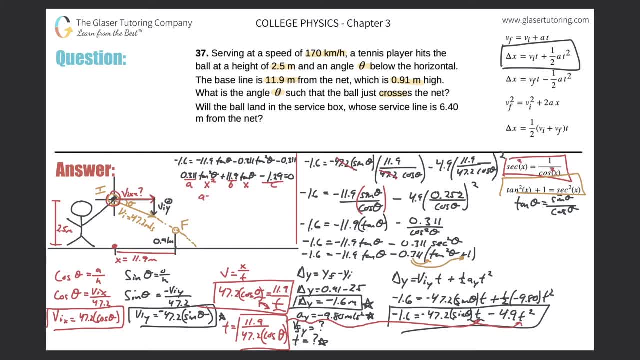 So I'm going to plug it into my calculator at this point, All right, So just know that the Um, That my a value here is 0.311.. My b value here, just so we're clear, is 11.9.. 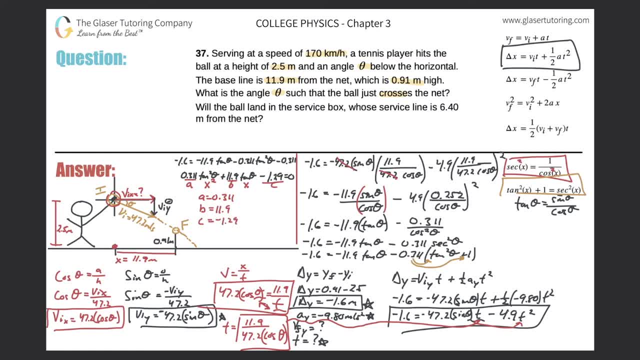 And my c value here is negative 1.29.. All right, So when I now use those values, let's see what I get. So I'm going to go to the calculator program. You can also graph the thing and then figure out where it intersects the x-axis. 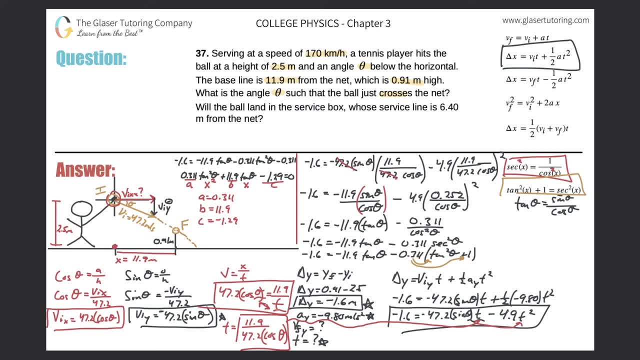 That's fine too. Point 311 is the a, Okay, 11.9 is the b And c is negative: 1.29.. Okay, All right, So I get two values. You can basically reject the negative value. That's not going to be important. 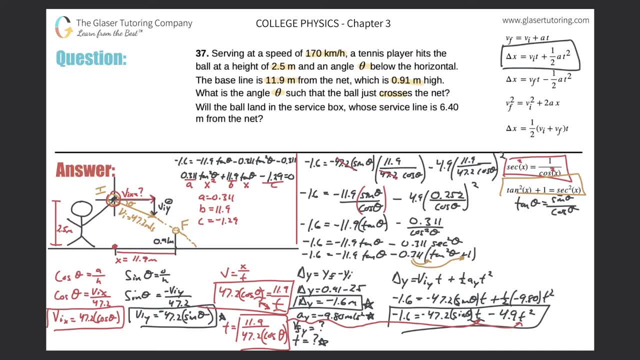 All right. So what we have here is: So let me write this. So now I have, I found that x is equal to, So x will be equal to 0.108.. Now, remember That was x. Okay, But what did my x represent in the problem? 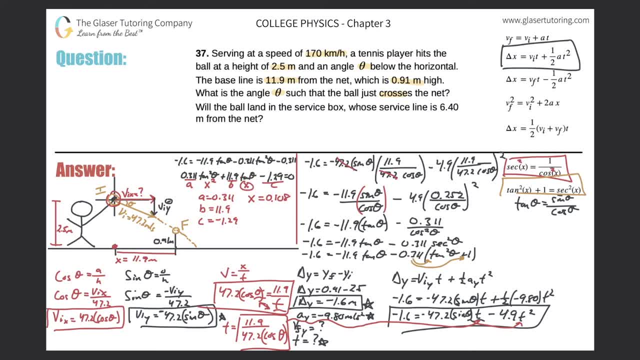 Well, my x here represented tan of theta, Right. So I can't really just write x here. I got to really really write tan. theta is equal to 0.108.. Now how do you solve for theta? Just do the inverse tangent. 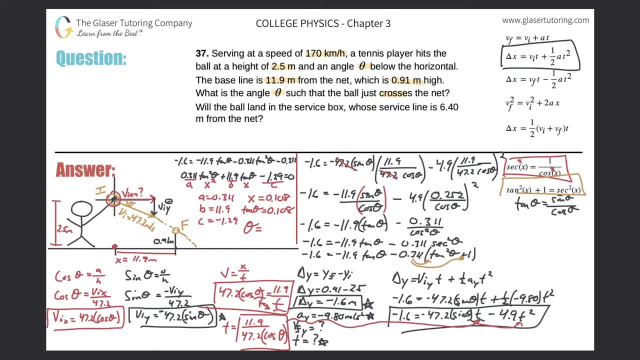 Oh my goodness, Finally, Hopefully we reach the promised land. Let's see Second tan of 0.108.. That looks pretty good to me. Looks pretty much on point. So now the theta value here is going to be 6.16.. 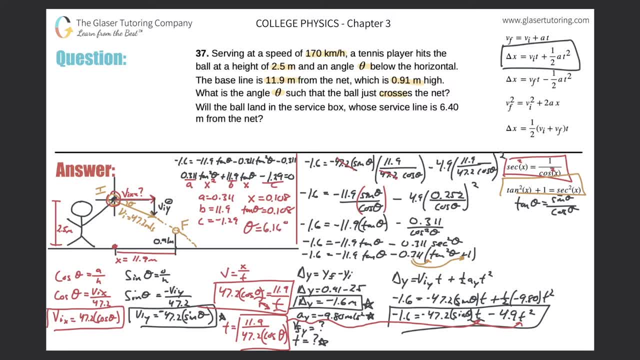 All right, So 6.16 degrees? Oh, All right, Man, That's a long problem and a hard problem, But we got there. Now I think I may have added one significant figure in here, So maybe the answer should be 6.2 degrees. 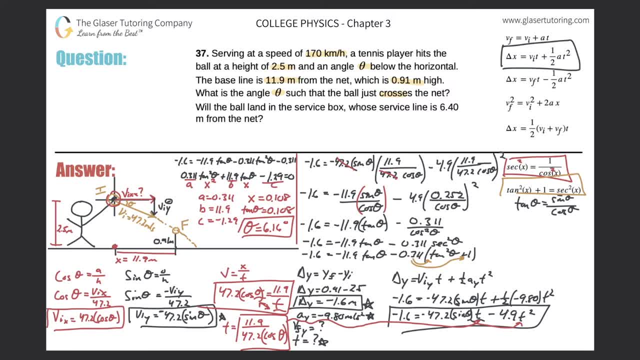 Technically, But at this point who cares? All right, So we got that. So we know our theta value now is 6.16 degrees. Now what are we going to do? All right, So we found that. now it asks us: will the ball land in the service box? whose service line? 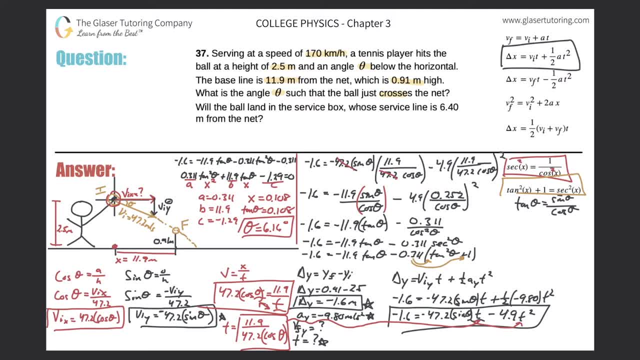 is 6.40 meters from the net. So, basically, what they're telling us is this: that there's a service box here- If you're familiar with tennis, Right, There's a little service box into all right and they say that it's distance from the net is going to be let. 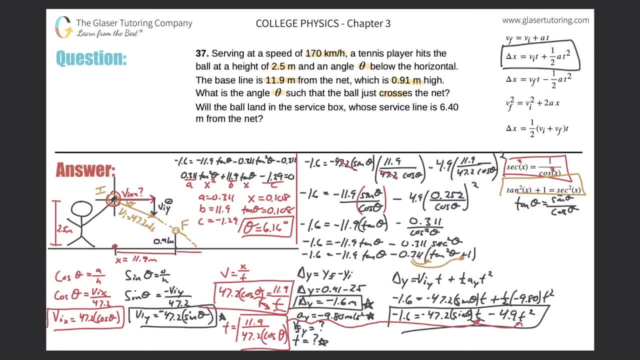 me make it a little straighter. its distance from the net is going to be- why didn't that come out straighter? there we go. its distance from the net is going to be six point four meters, so this little piece right here is going to be six. 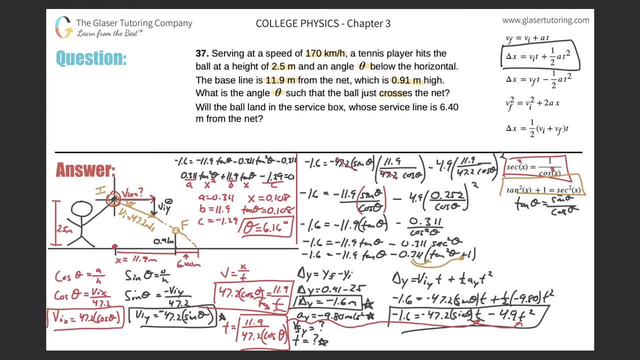 point four: zero meters. okay, so we have to figure out, well, whether it will land in the box or not. so the first thing is what I want to do: remember we all we found was the angle. we never really found the initial velocities yet in the X and the Y frame, and we're gonna need that in order to calculate our answer. so 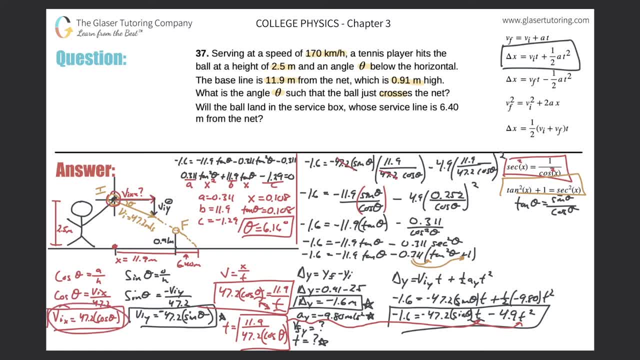 please bring your attention down to the bottom left of the page. here are my formulas right that I used before. I didn't actually have a value for the initial velocity of X, but guess what I have now. I have my theta. so now I can go and plug it in right and find the initial velocity of X, and then I can. 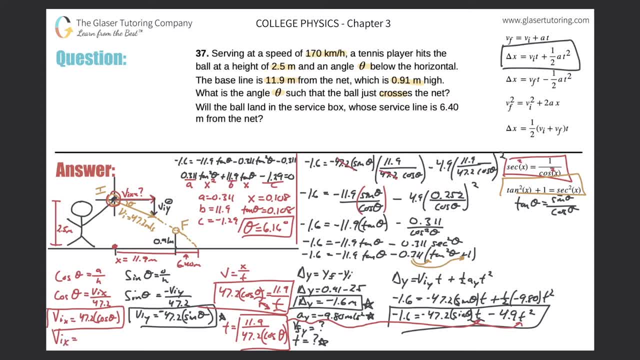 find the answer. so the initial velocity in the X direction is going to be so simply do forty seven point two times the cosine of the angle. we found six point one, six degrees, and that works out to be forty six point nine. right, so we get a value of forty six point nine meters per second. that's the X initial. 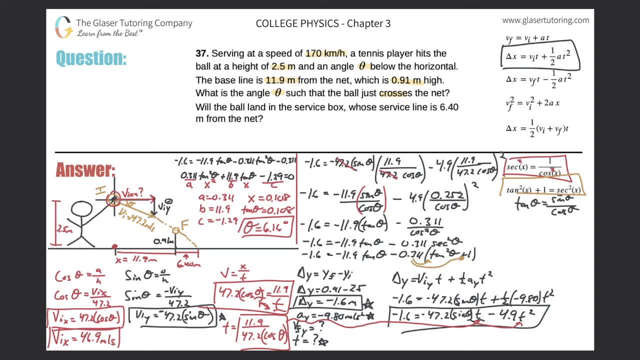 X velocity. why don't we do the same for Y, since we're right here, so the same thing happens. if we do the same for Y, since we're right here, so the same thing for Y, now, right next to it. simply take negative forty seven point two times the. 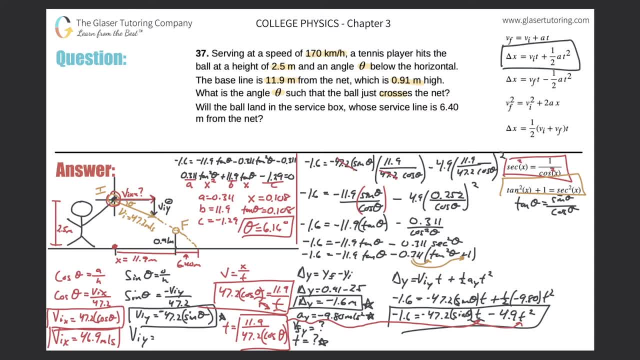 sine now of six point one six, and we get a value of negative five point oh six. so negative five point oh six. all right, and that should make sense, because it's in the negative Y direction. so we're good here, all right. so now how do I figure this out? whether it's gonna land in the box? 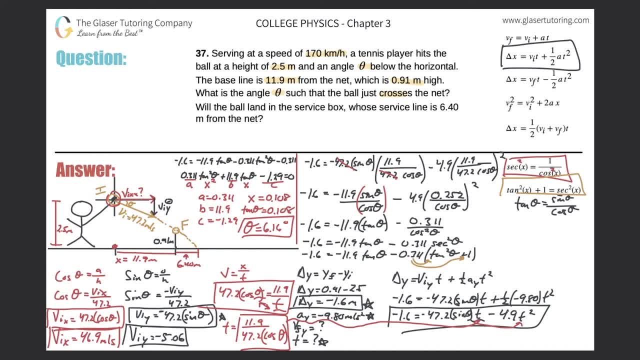 or not. well, the important thing here is: I need to know the time. I gotta figure out the time the balls in the air, all right, in order for me to answer the question. so what I want to do is calculate the time ball is. my writing is terrible. ball is in the air, okay. how do we do that? well, it's easiest to do this. 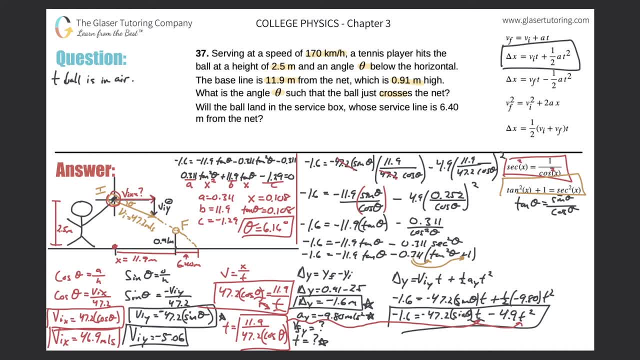 if we- let me think about this actually. well, we could do it either way. no, no, no, actually, no, no. I have to do it in terms of the Y direction. all right, because it's in, it's in freefall accelerations pulling down on it, so we're gonna be. 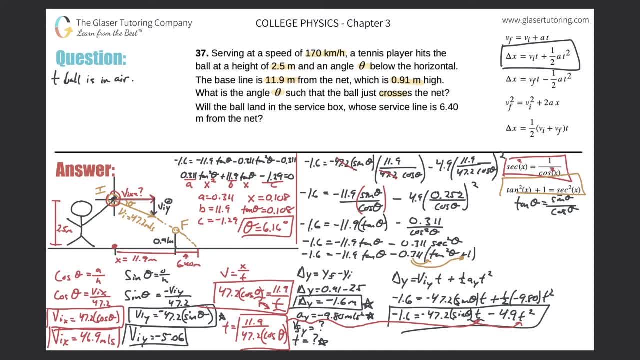 able to figure out the time from the Y direction. all right, so let's let's list the things we know. we know that the initial velocity in the Y direction is going to be negative. five point, oh, six. okay, we also we don't know the final velocity in the Y direction. right, we don't know the velocity which will hit. 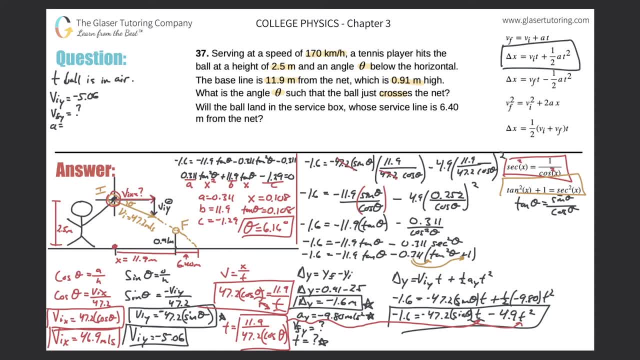 the ground with. we do know the acceleration, though, and the acceleration should be negative nine point eight oh meters per second. we also know the total height that the ball, or the right the ball- will travel. the total height the ball is going to travel when it hits the ground right is going to be two point five meters, because, essentially, my 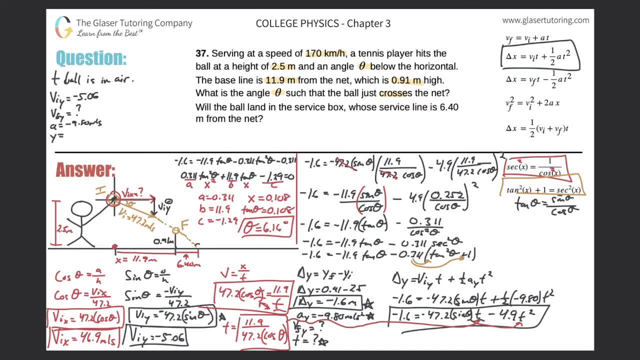 frame now the initial frame is still here, but I shifted now my final frame to the end. so the height differential now is negative. two point five: why is it negative? because it's going starting high and ending low, so it's traveling in the negative Y direction. so now I should have enough. I need in. 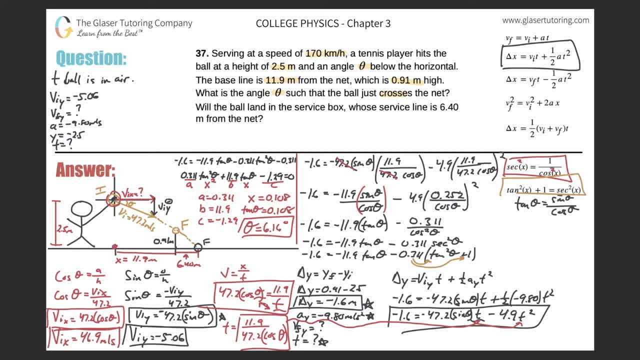 order to be able to calculate the time, in order to be able to calculate the time, in order to calculate my time. okay, so? yeah, let's do that. okay, so now what we need to do is what formula? sorry, I just got distracted- we have to select a. 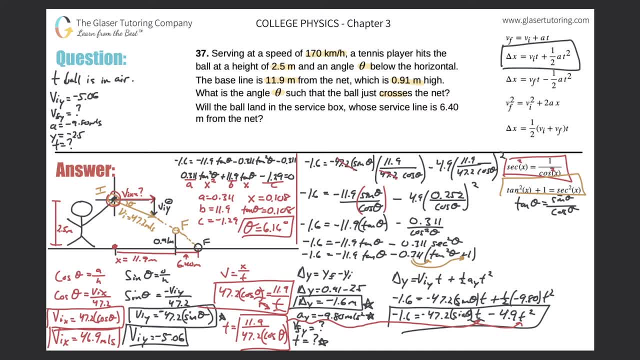 particular formula to use here, and it seems like we're going to be using- yeah, we're gonna be using number two again, okay, so I think we're gonna have another quadratic, but we're gonna do that quickly, all right. so so the formula for the exotic oval is this: is only: 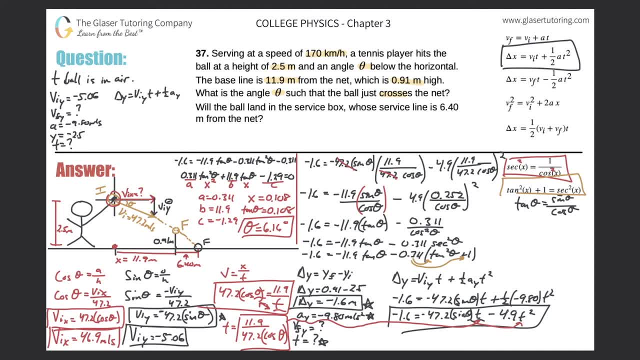 value being that you can take this arising from the derivative of exist, from themomenth one and depending on how long that Cears and evenings. so let's just bring everything on over to the left hand side to make the coefficients positive. so now it should be 4.9 t squared plus 5.06 t minus 2.5 is 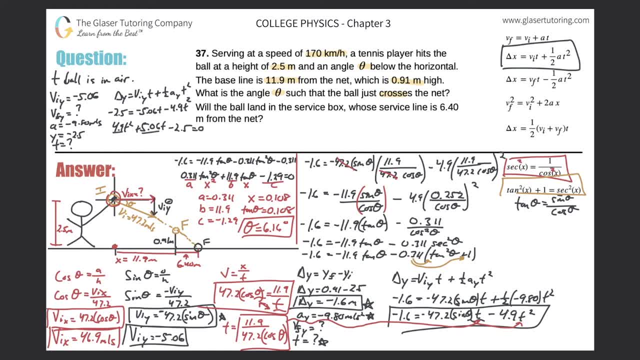 equal to 0. so there's your, here's your a, here's your B, here's your C, and now you can plug it into the quadratic again. I'm just going to solve now using the program here in my calculator. so the a value is 4.9, the B value is 5.06, the C 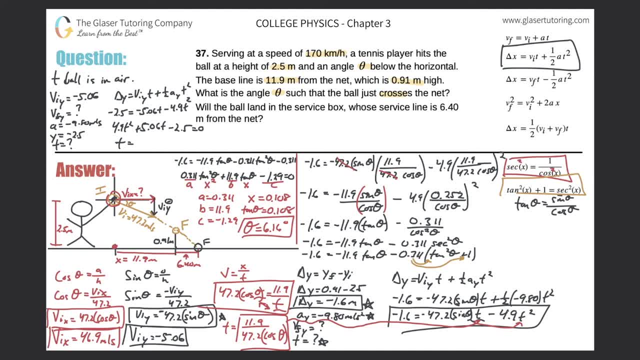 value is negative 2.5, so we get a time value. ignore the negative time. we don't have negative time here. so now it's going to be zero, point three. six, five, three, six, five seconds. that's how long the ball will be in the air. okay, now. 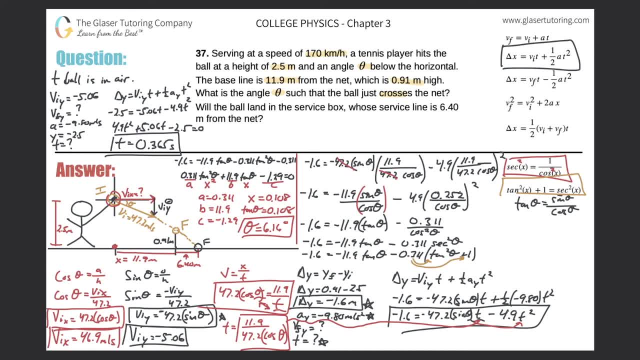 what do we want to do? well, we want to see whether the ball will now travel over to the other side of the table, and we want to see whether the ball will now so bring your attention to the picture. we want to see whether, how far in the X. 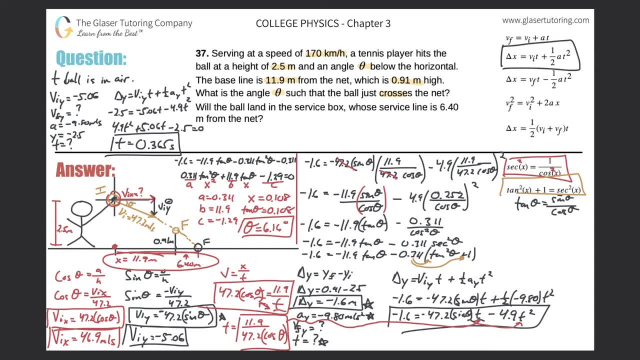 direction the ball will travel. if the ball travels in point three, six, five seconds, if it travels longer than this service line, meaning if it goes over here, well, bad serve. but if it is shorter, if it lands here, let's say if it's shorter than this distance, then we know it's going to be good, we know it's. 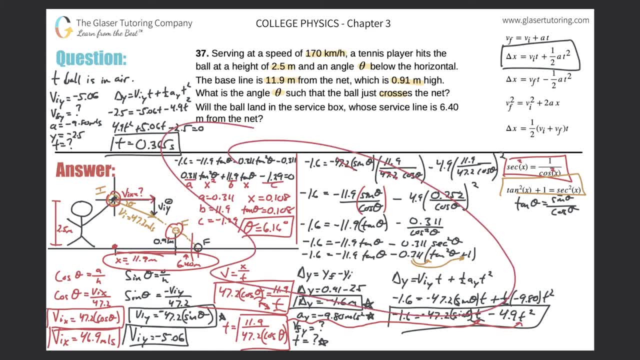 definitely going to go over the net, because that's what we did over here, right? that's the craziness we did over there, so we're good, right? so let's try to figure that out. so let's figure out how far the ball goes in the X direction with this time. how do we do that? 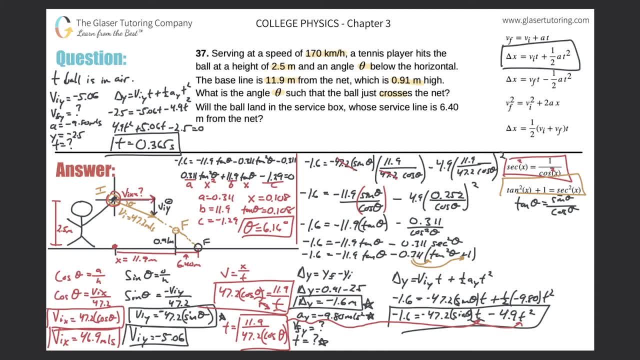 well, remember, we already have this particular formula right. we know this formula: V is equal to X over T. ok, so we. so let me write this here: the average velocity in the x-direction should be equal to the X displacement over the time. so what is the average velocity in that transaction? well, it's never going to. 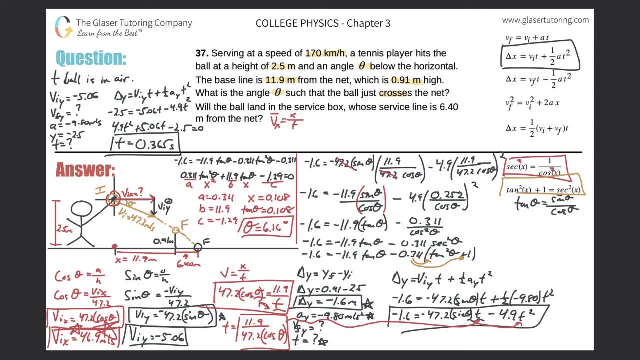 change. it's always going to be the bottom left-hand corner, 46.9 meters per second. so this is 46.9. okay, 46.9 is equal to then X, because I'm gonna solve for the displacement. I know the total distance here, but what I want, 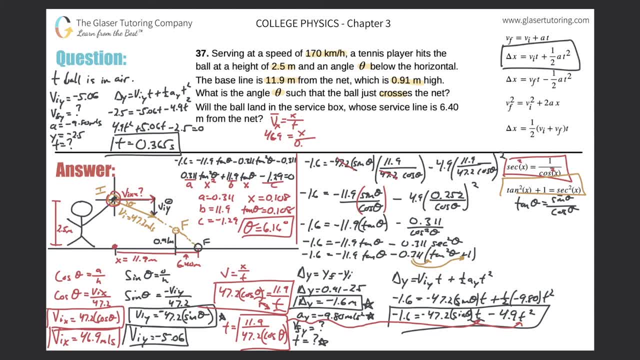 to do is: I want to see how far it will travel, given the time that it will be in the air. 3, 6, 5. so now, when I just do a simple cross multiplication here, I get four, forty, six, point, nine times point three, six, five. so get a value of seventeen. 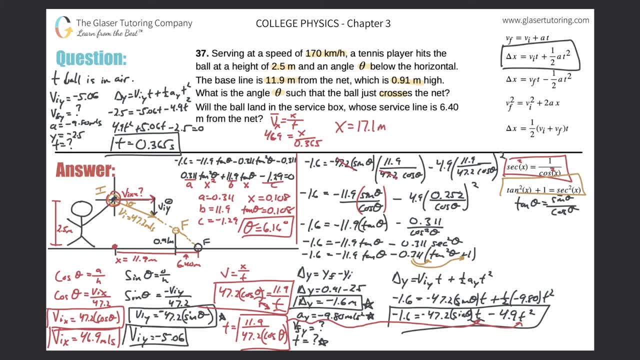 point one. so this is seventeen point one meters. all right, that's how far the ball will actually travel. this is the actual, actual range. okay, but what's the maximum range that it could have traveled? remember, it's it from the point of the balls release it had to have traveled. 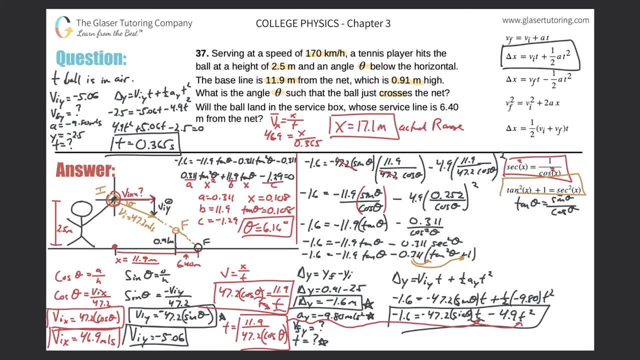 eleven point nine meters to the net, and then it was allowed to travel a maximum of six point four more meters right until the end of that service line. if it traveled more than that, it's no good. if it traveled less than that, it's good. so let's calculate the maximum, okay? so this should be easy. so I'll call it X max X.